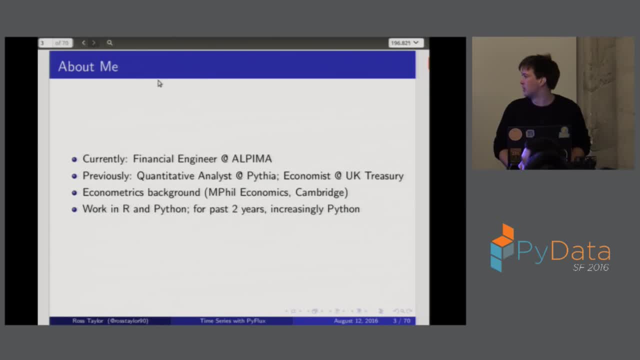 So about me. I'm currently a financial engineer at Alpima, which is a new financial advisory startup based in London. I've previously worked as a quant looking at sports prediction markets, and I also worked as an economist. My background's in econometrics and stats and in terms of languages, I used to work a lot in R and now I'm increasingly Python. 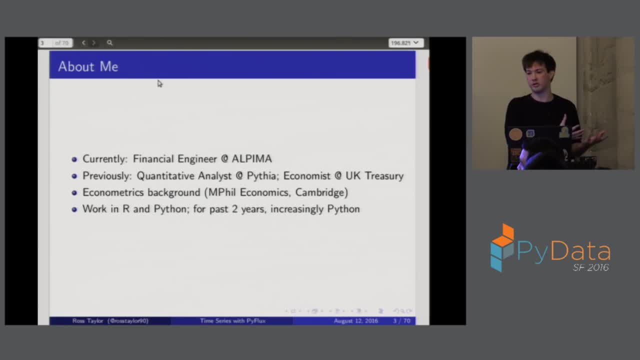 I can say from a personal development point of view, it's been really useful, because I'm from a research-based thing and Python's made me think more about the quality of code and software. I'm not quite there yet, but you know it's been very, very helpful to me. so 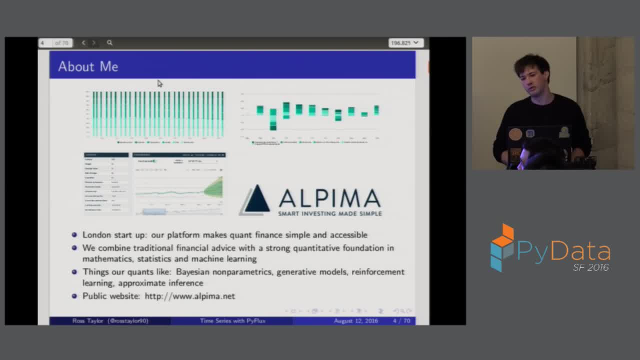 And just a quick word about my company, very quick. So yeah, we're a financial advisory firm and what we try and do is that we try and combine traditional advice with, like, a strong quantitative foundation in stats and machine learning. 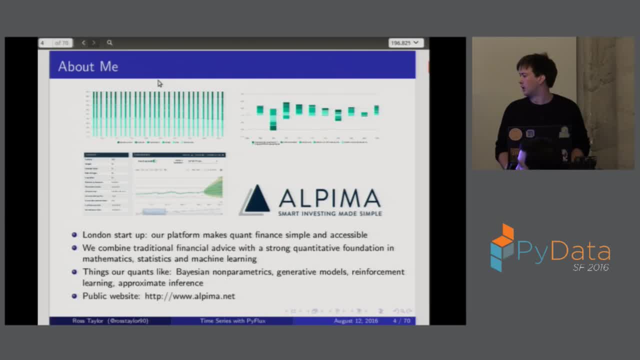 So we do quite a lot of cool stuff, but we're kind of aimed at institutional investors. But we are looking to have like a free website which allows you to build portfolios and stuff, you know, for the general public soon. 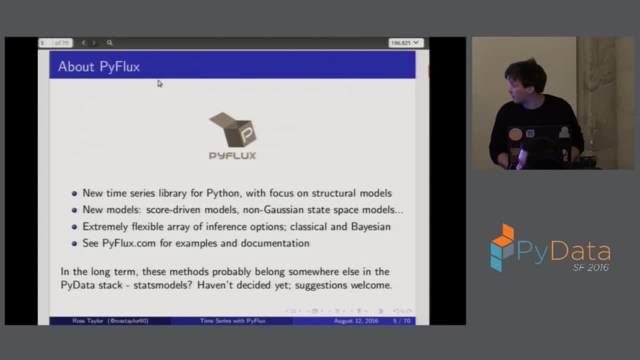 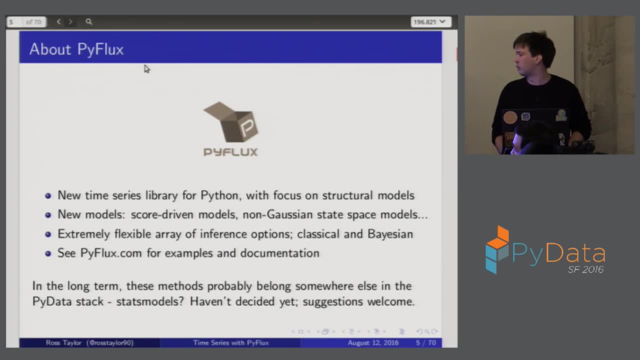 So stay tuned for that And about Pyflux. So this is just a personal project that I've been working on. I'm not going to lie, there are a lot of like selfish reasons. just I wanted like more experience with, like working with software. 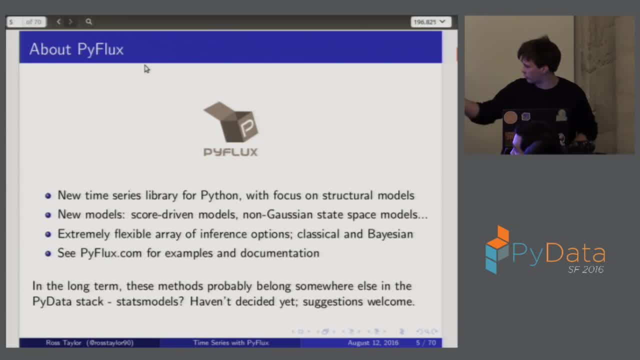 But in terms of what it like can give you. there's some new models, one of which I'm going to cover today- score-driven models and another model type non-Gaussian states-based models, which are quite useful. It's also quite original in the sense that a lot of time series like packages and libraries right now. 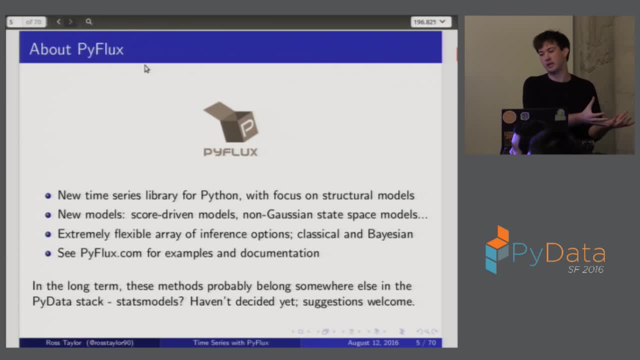 they kind of force you to use one method of inference like maximum likelihood or, you know, one might be a Bayesian approach on something, because I've tried at least to allow you to do like both for most of the models. 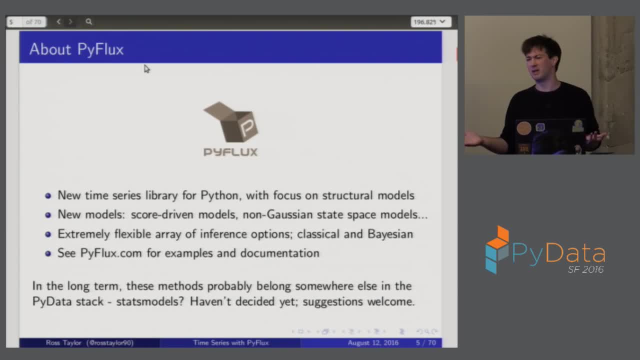 Having said this, like to be honest. like most of these methods, it probably belongs somewhere else in the PyData stack, like probably like stats models or something. The only reason why I haven't quite got to the stage of maybe trying to like integrate that into stats models is that 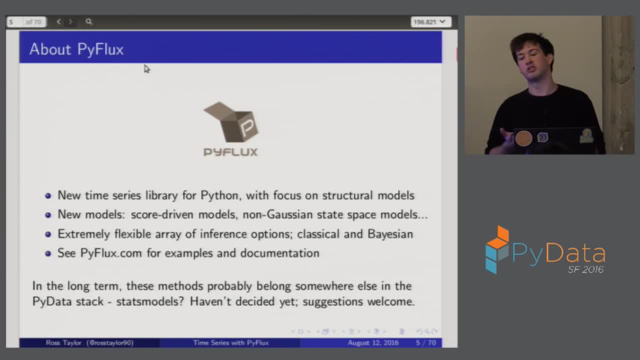 stats models, portrays itself as like frequent tests and like. so it does things like maximum likelihood and moment things, And I kind of like to maintain the flexibility. So I haven't quite worked out where it fits yet, but I'm open to suggestions where you guys think these methods should go. 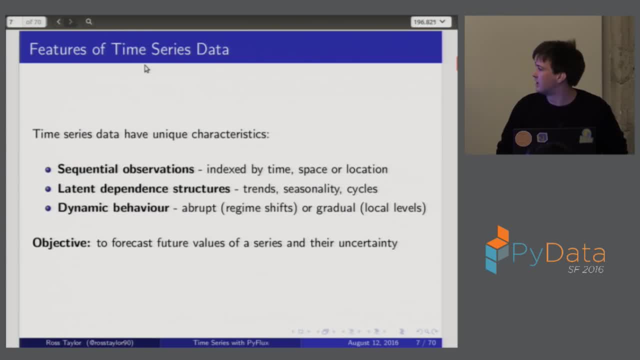 So introduction. So this is kind of obvious, I guess. but there are unique characteristics you should be aware of. So time series is sequential. You can't like shuffle the deck, so to speak, of the data, And we're also interested in these latent dependent structures. 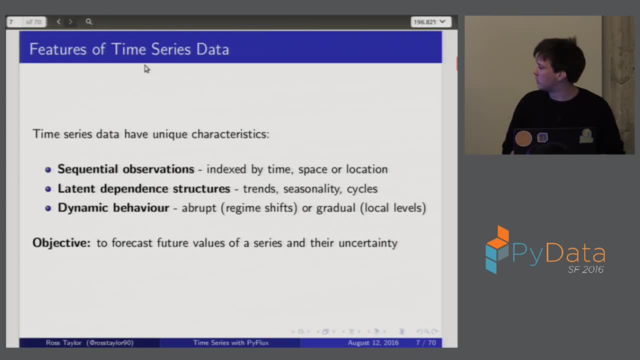 So trends, seasonality, cycles, And in particular we're interested in dynamic behaviour which could be abrupt, So regime shifts, which are quite popular in finance- or gradual, So you might have like behaviour that just changes over time, gradually. 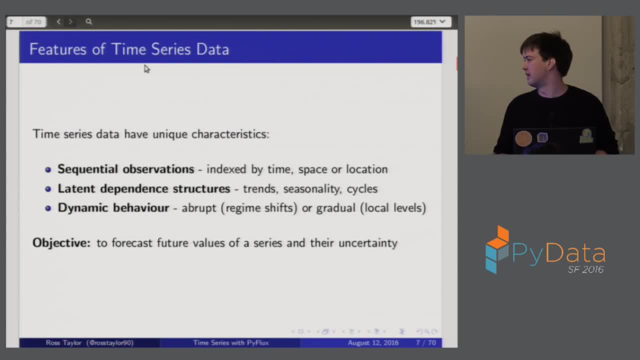 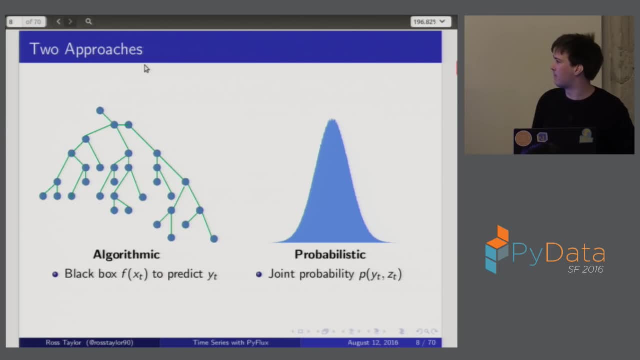 But overall I guess you could characterise what we're doing. We're trying to forecast future values of a series and the uncertainty associated with it. Now two approaches, So this actually is maybe a bit deceptive because there's some overlap. 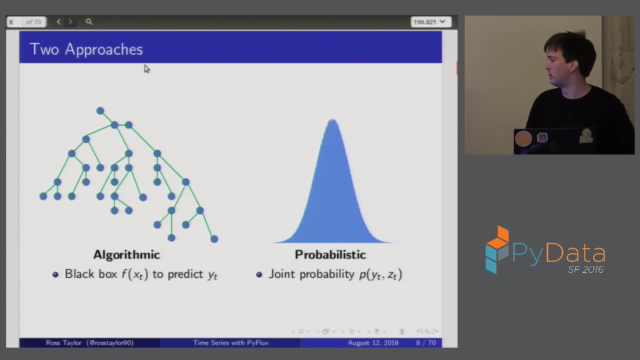 But I guess this permeates a lot of perhaps the talks you're going to see at this thing as well. So the algorithmic approach focuses on trying to get like a really tight, like black box nonlinear function. So you're talking about things like SVMs, neural networks, random forests, that kind of stuff. 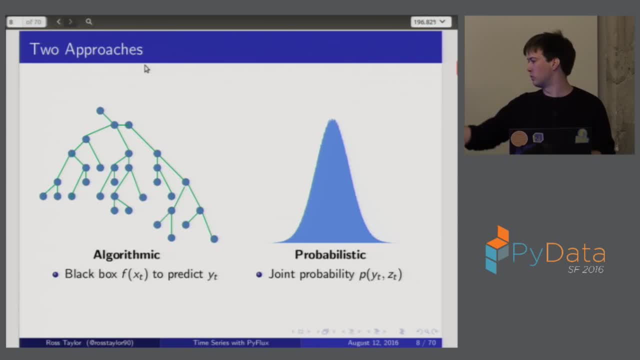 Whereas the probabilistic approach has been more academic, but it's kind of. you're looking at this joint distribution here. So yt is your data and zt is some latent variables, And I'm going to focus on the one on the right today. 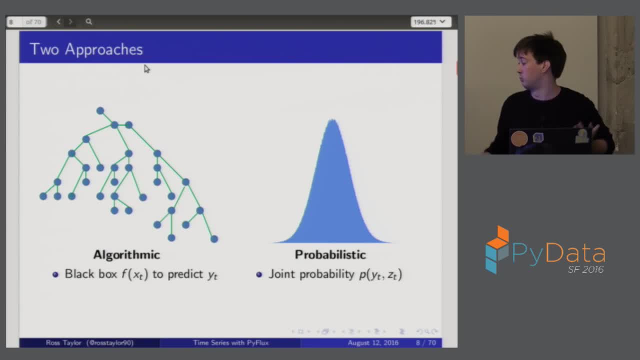 But it's worth, You know, worth like being aware of the overlaps, For example, neural networks, which are all the rage these days, Something like dropout, for example, that actually has like a probabilistic interpretation. What you're doing. when you're doing something like dropout is you're actually doing approximate integration. 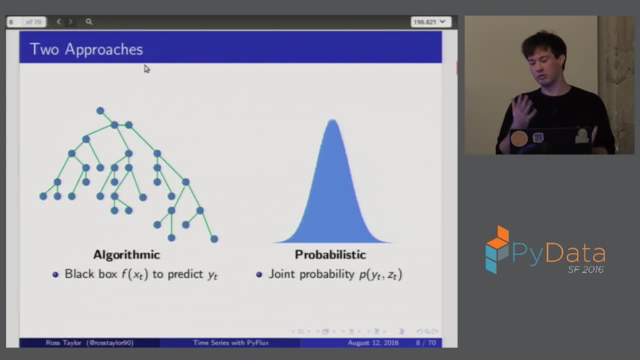 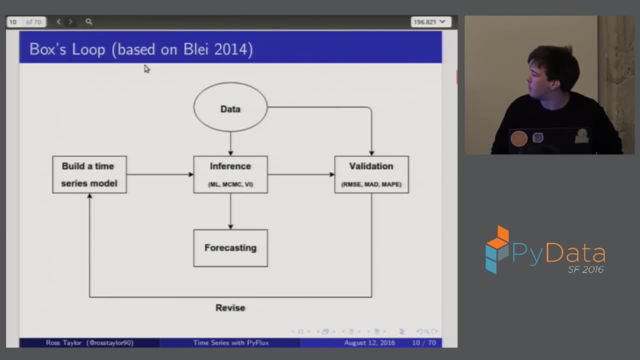 So you're basically doing something like approximating a Bayesian model. So I think it's interesting to look at that, those kind of overlaps, if you haven't had a chance to yet. So that's the focus Boxes loop. So this is something I saw in a paper by David Bly a few years ago and I quite like it. 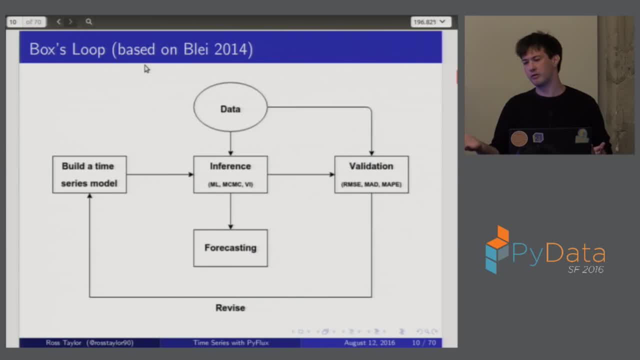 And I saw it more recently In a package called Edward- you might have heard of it's- by Justin Tran and he's advocated this boxes loop thing And I quite like it and I think it's quite good for time series. It's not like a true thing. you can't really like validate this as like the best way. 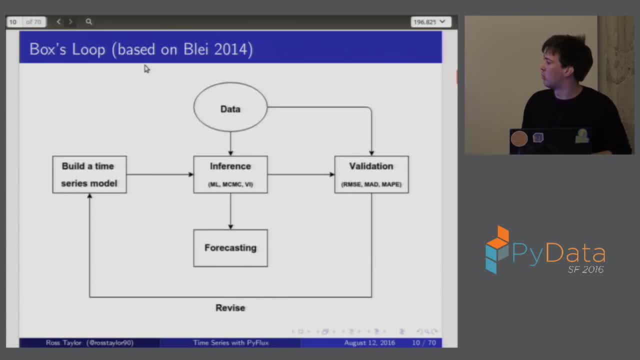 to approach something, But I think it's a useful like set of heuristics. So what we're interested in doing, we build a time series model, we perform some kind of inference. so maximum likelihoods maybe MCMC, variational inference. 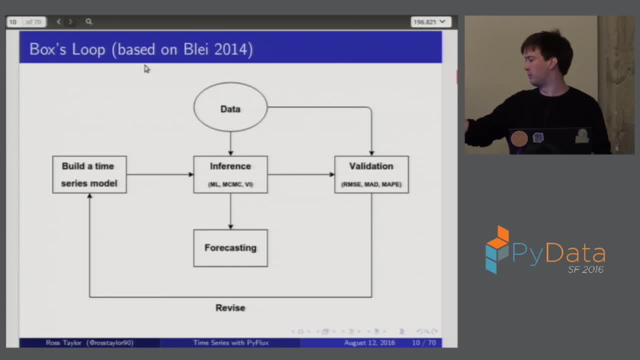 We look to validate our model. So in time series that's a lot focused on, say, your out-of-the-box model, For example, performance like mean, squared errors and stuff, or maybe just looking at the fit. And then, once you've seen that, you have an idea of the weaknesses of your model, when 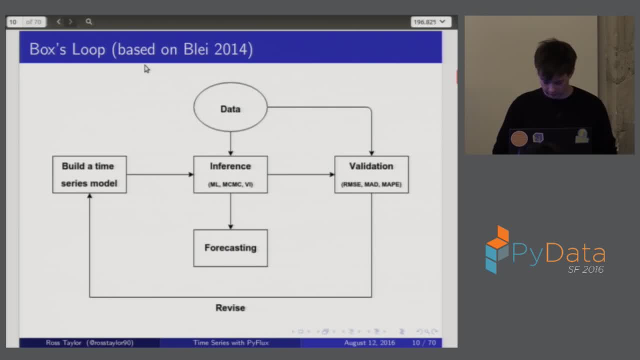 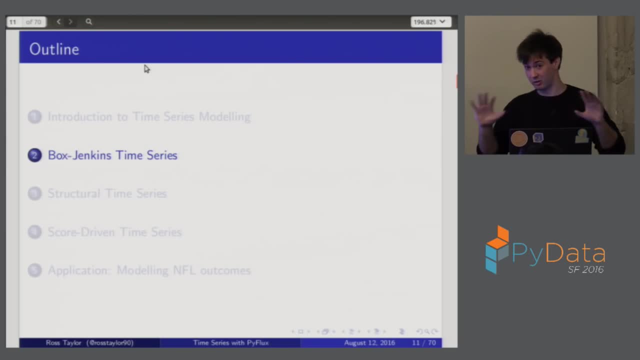 you go back and revise and when you're happy you can go ahead and forecast. So, Box Jenkins, I'm going to cover this very briefly because there was a great tutorial yesterday, so I'm assuming the guys in the room at least are all experts on Arama models. 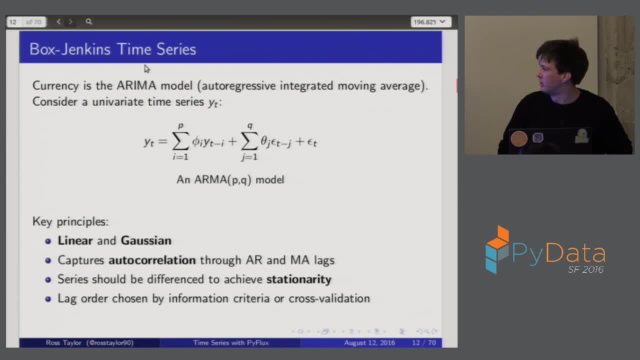 But I'll just like focus on the high-level idea behind this. So this is the currency of this philosophy: the Arama model. So what you're trying to do here is essentially capture autocorrelation in your series, At least just by these lags. so you can see these two sum terms. 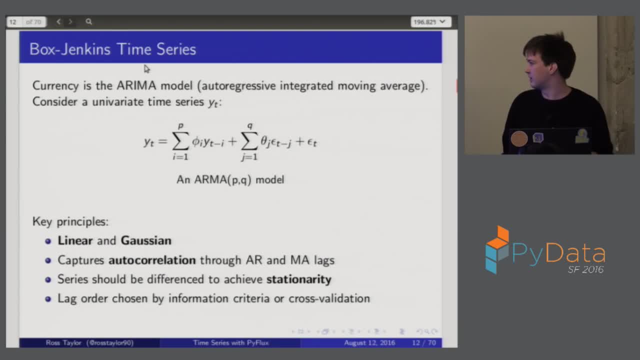 So auto-aggressive and moving average lags. So the key principle is: it's linear, so you can see the additivity, and it's Gaussian, so this error term here is Gaussian. So the idea is that you basically difference this series to try and get a stationary series. 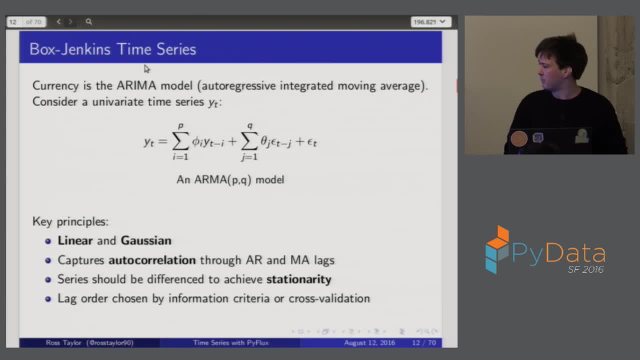 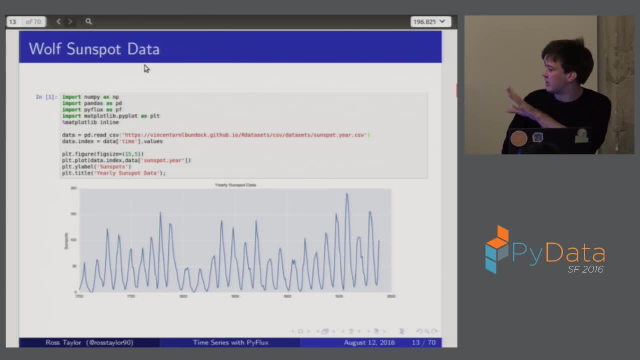 and then you try and choose the lag order and then you go ahead and forecast. I don't want to go into detail on this, but I'll just, perhaps, like, maybe, just like blast one myth that's sometimes heard. So this is some data, sunspot data, sort of common time series thing. 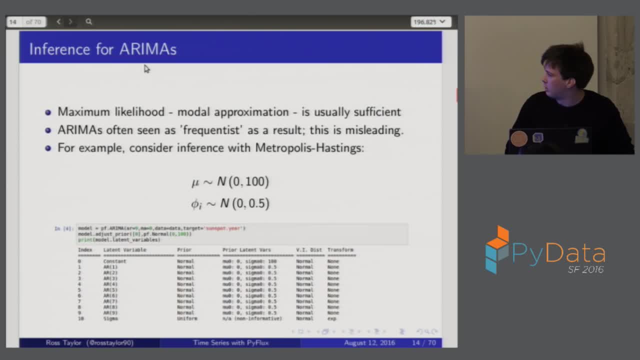 As you can see, it's very cyclical And this is the room I So a lot of people I've seen on like blogs and stuff. I don't know why, but, like some say, like Aramas are frequentist. 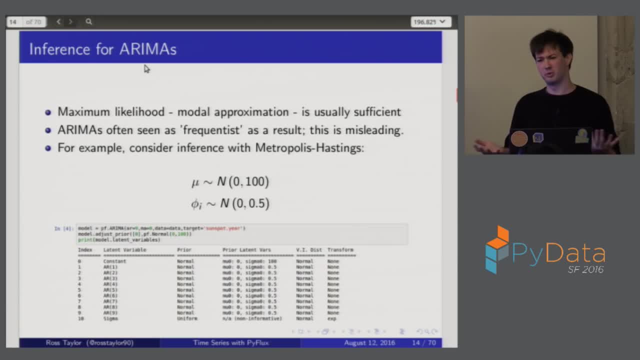 But I guess one point I'd like to get across- this is very general- is it's like models, in my opinion at least, aren't frequentist or Bayesian. Like a model gives you a likelihood, You can augment a likelihood with priors and do Bayesian inference on it. 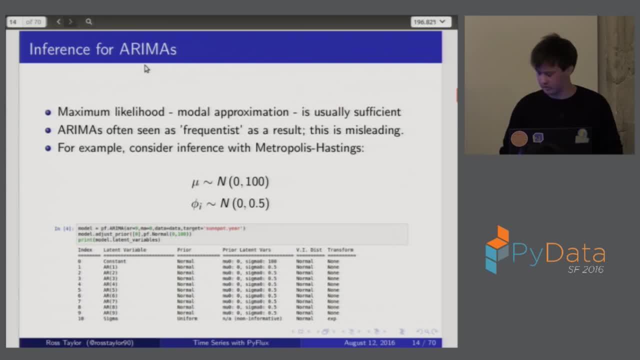 So calling a model Bayesian or frequentist is in my opinion. it doesn't really make sense. So just for the hell of it, here's an Arma 9 model: Nine autoregressive lags, And I'm just doing metropolis hastings. 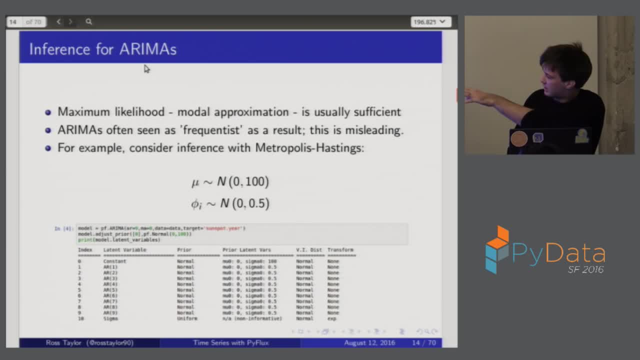 So there's a constant which is a set of quite large variance parameter there. So it's weakly informative. And the AR terms- I'm just assuming this is normal prior and I've basically set the variance here. So it kind of discourages terms which are like above one in absolute value. 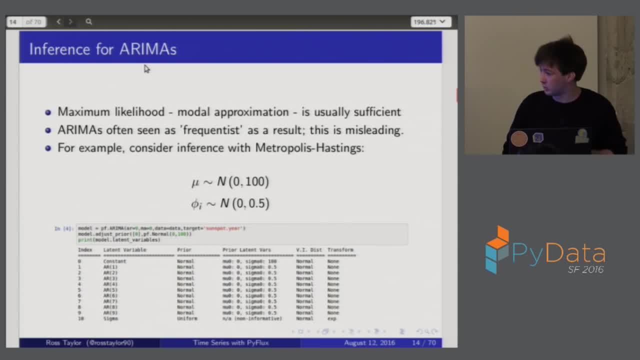 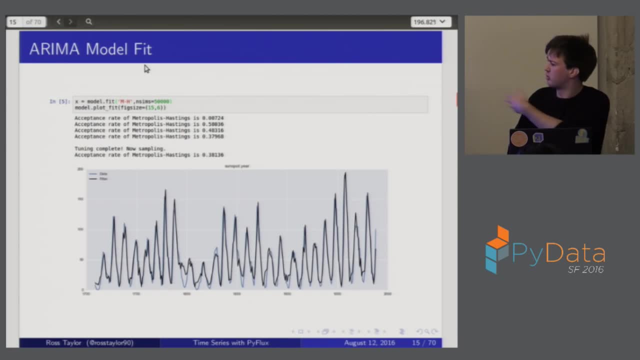 Because that tends to be associated with more like non-stationary series. Not necessarily, but yeah, So that's just an example, using the Pyflux library, So you can see, and this like carries through to other models. 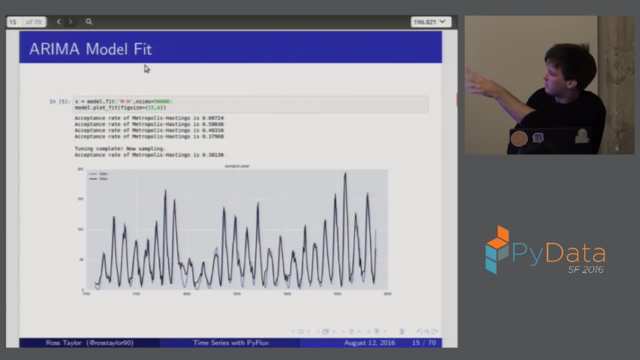 To be honest, if you're doing Armas, you're not going to want to use this library, probably. But the point is that, like the model fit here, you can choose whatever you want. So here's like metropolis hastings. 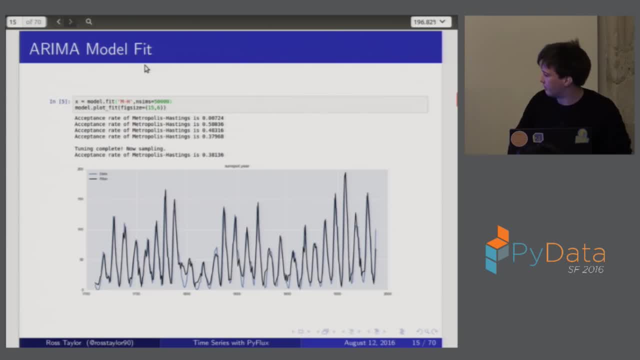 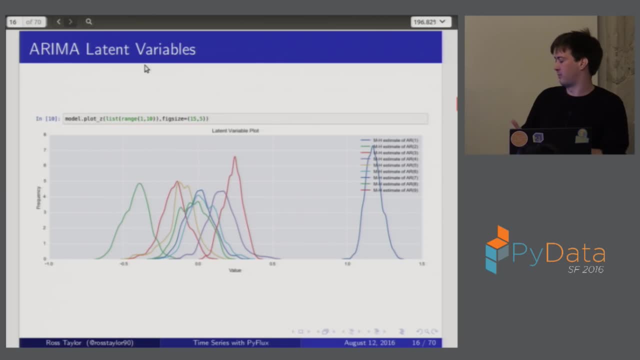 I've just done like a long chain And then I've just plotted the model fit And you know it's a fairly good fit within sample And you can also plot relation variables. So a lot of statistic packages give you like tables. 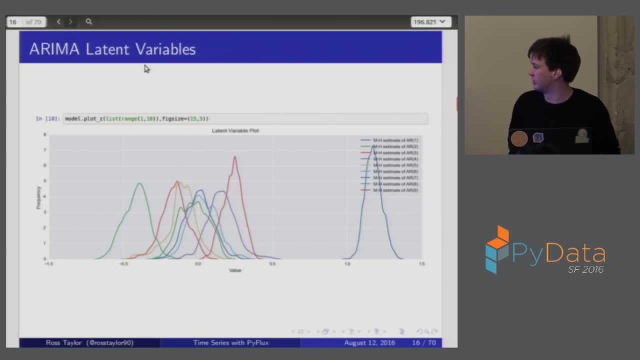 And I quite like the idea of graphing stuff because it makes people think about uncertainty. So this is from metropolis hastings. You can see it's a bit wiggly because of approximation, But you can see where the uncertainty is in these AR parameters. 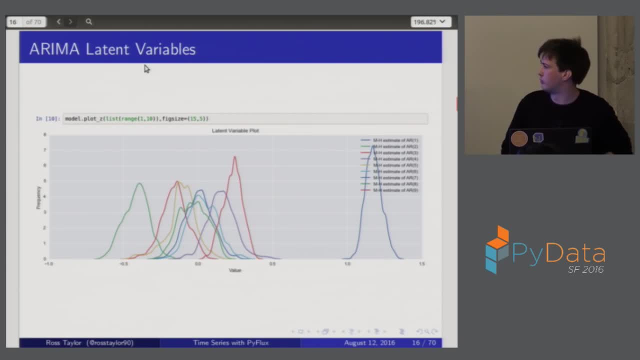 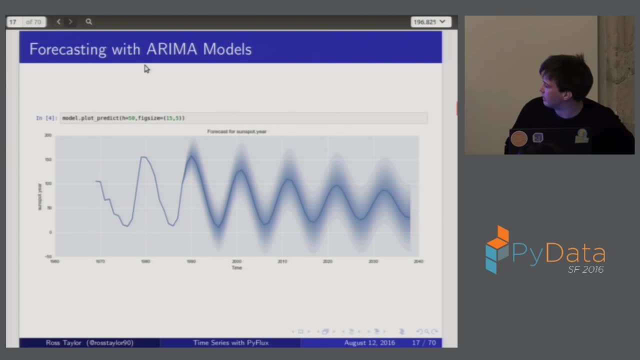 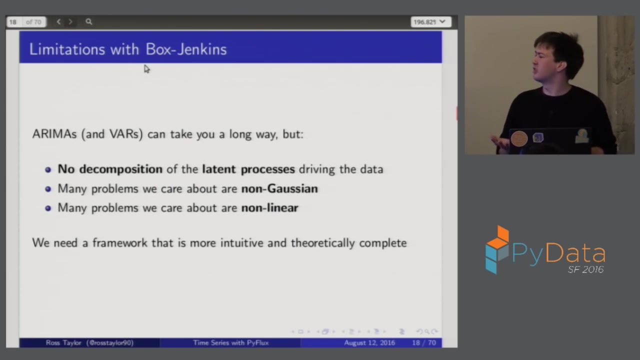 And Z is just a term for latent variables or parameters And forecasting. You know it looks very nice, this sunspot data It's. you know, very easy here as well, The limitations. So these types of models can take you a long way. 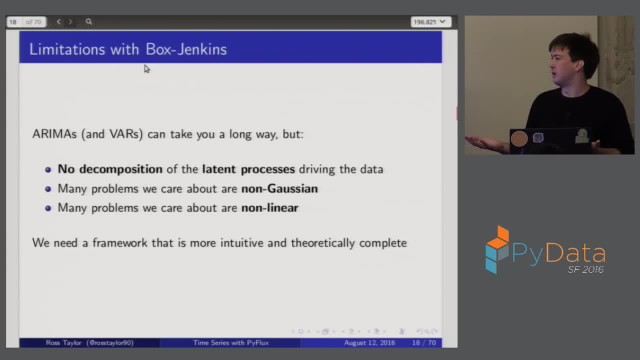 And if you're like first approaching a time series, perhaps you're going to do this kind of thing. But to be honest, I don't really like it from a theoretical perspective, because there's no decomposition of the latent processes from the data. 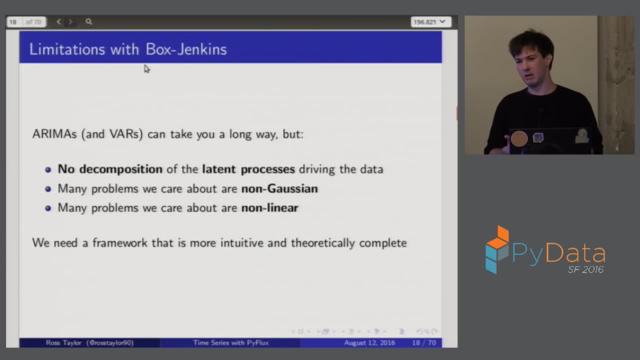 That's a bummer. I'm a bit wordy, But what I mean by that is we have some kind of idea that we're going to fit a series with like AR and MA lags, but we're not really directly like capturing things like trends. 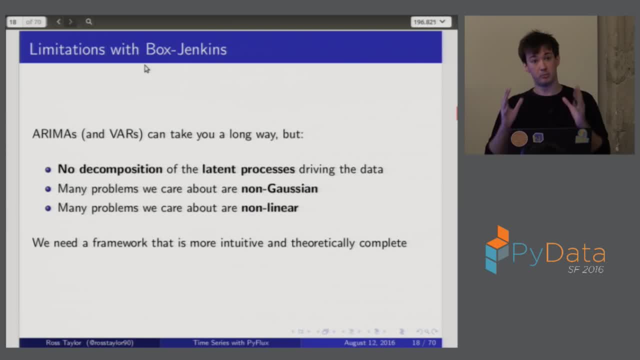 cycles. Ideally, what we'd like to do is actually get them directly out in the model by specifying the model so it has these components and then we extract it, rather than just fitting lags and like assuming that we're capturing these features. 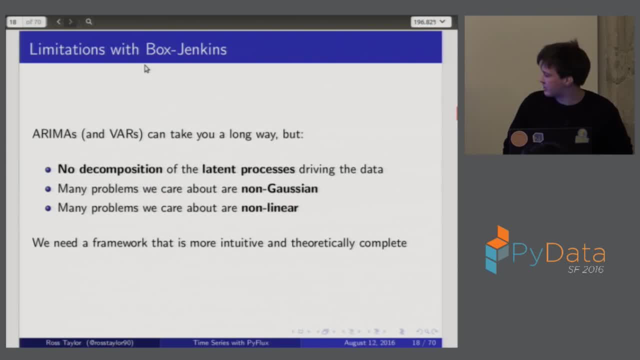 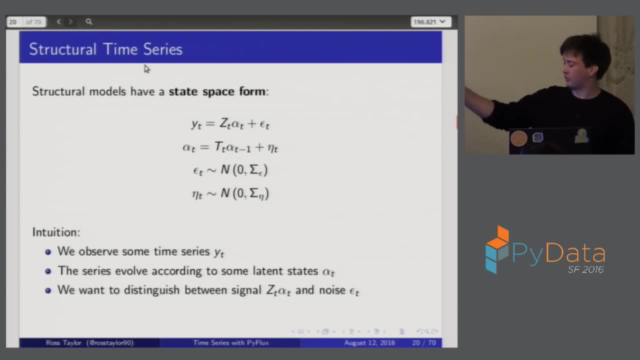 More generally, many problems we have are non-Gaussian and non-linear, So we need a more intuitive and theoretically complete framework, And this is what's called structural time-based. So this I'm going to explain it intuitively. so what's going on here? 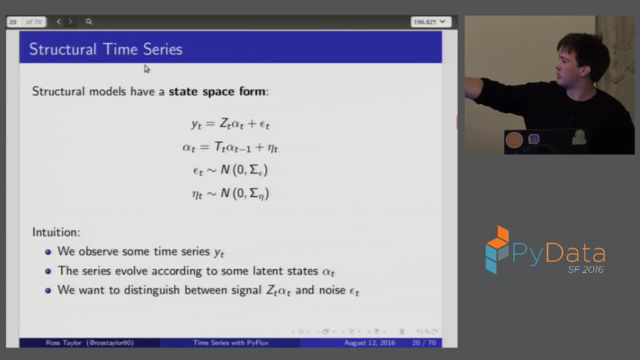 Why Imagine this is like a univariate time series, Why We assume Y is a function of some unknown states. So, to give an example, imagine we have some tracking- you know tracking data on someone. Imagine this tracking data is a bit shit. 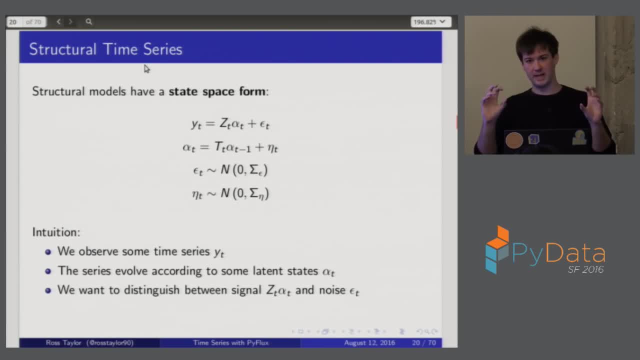 So, like in that situation we'd be interested in the state would be that we don't directly observe Where is the actual position of this person, And we're going to get measurements in and we want to filter out the signal from the 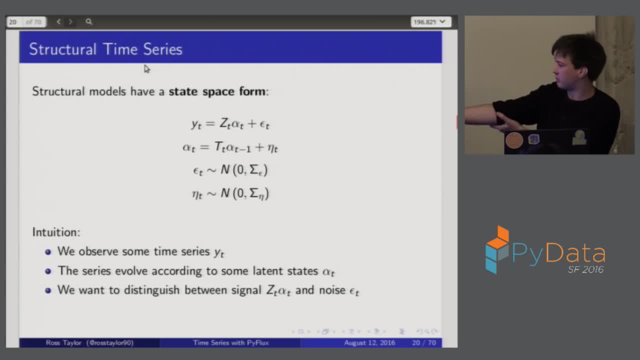 noise. That's the basic principle behind a state-based model. So we observe some time series Y, The series evolves according to some latent states and we want to capture this signal and this noise. So that's the state equation, there the alpha, and so it's like a Markov form. 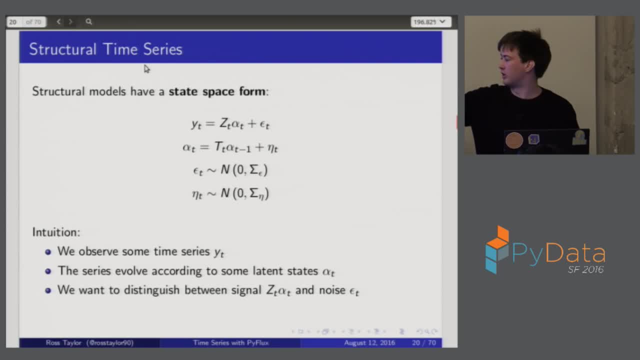 And that's the underlying thing we really want to get out of this. And Y is a function of this unknown thing, plus some measurement error. Does that kind of make sense? A good anticipation. we're going to come on to that, But before we do, let's think about the function. 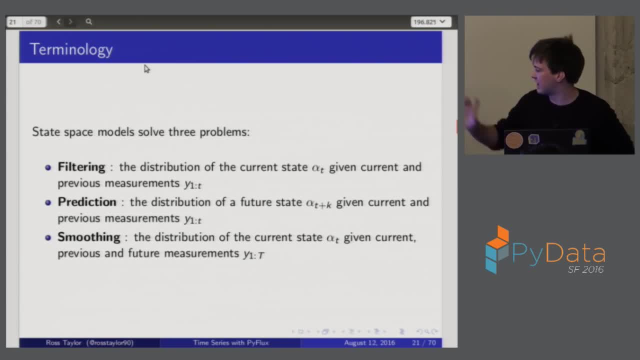 What's the function? Yeah, So we have some problems that this solves. And again, this is a bit wordy, but there are three things. Filtering is that you're interested in the current state. given current and previous measurements, You're interested in the present. 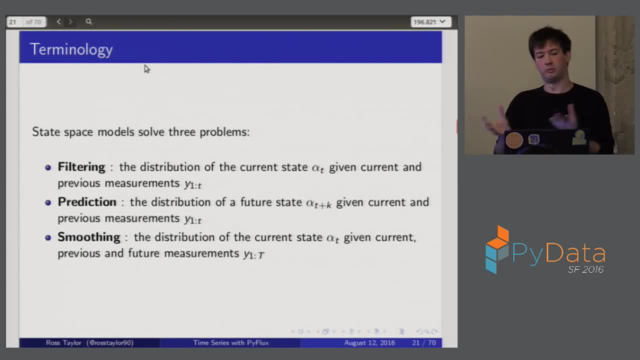 A lot of times for big data. you're interested with filtering because you don't want to have to store all the data in the past because that's a bit costly. Prediction is similar, but you're interested in future states And smoothing. is that you're interested in the past? 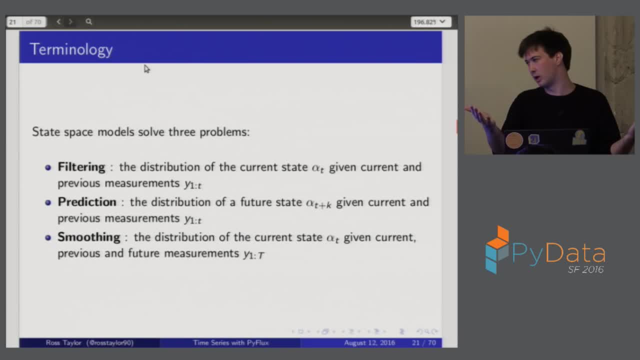 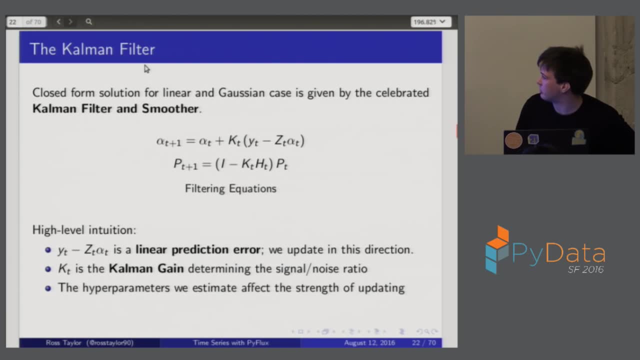 So if you want to know just what the true location of someone was 10 minutes ago or something, you're going to use future and past data, And this is going to come on to the case. So this is the Cameron filter, as you said. 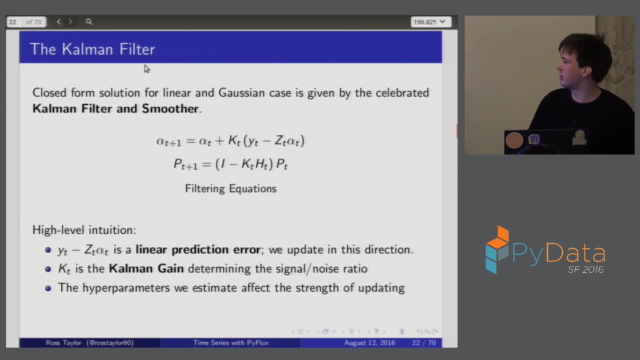 So actually for the formulas I showed you just two slides ago, there's a closed-form solution for this linear and Gaussian case and it's a celebrated Cameron filter and smoother. So the Cameron filter was actually developed in the 50s and 60s. 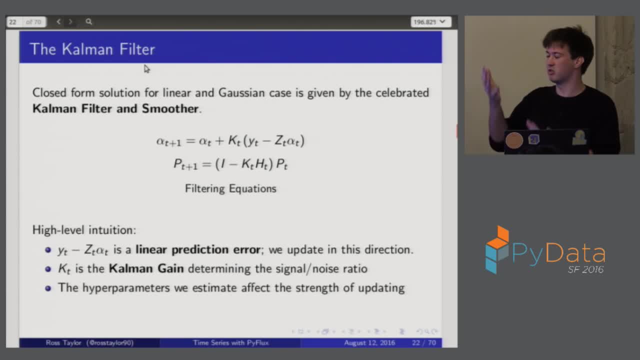 Its first use was actually, or major use was, in the Apollo missions, and what they were interested in is basically trying to get the land on the moon without it crashing or bouncing off, And they had noisy measurements. The history is actually quite interesting, because they actually considered using an 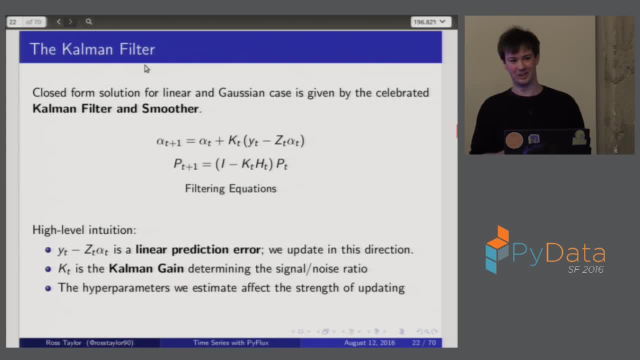 algorithm called weighted least squares, but that was too computationally intensive for the computers they were using at the time. So they ended up using a Cameron filter, because it's a filter and they don't have to store the past data. So it's quite interesting. 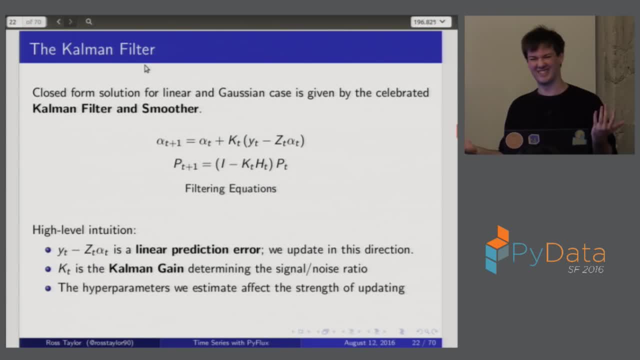 But unfortunately I work on planets so I don't get to do useful stuff like landing on the moon, however useful that may be. So high-level intuition. So alpha again is the state right And you don't have to worry about the variance term p, but that's basically your idea of 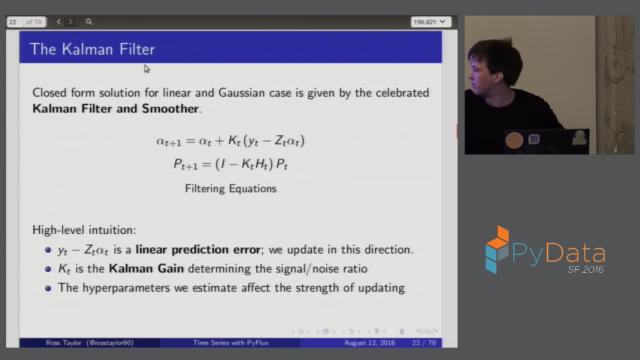 uncertainty. And so what's it a function of? So this term here the yt minus ct alpha, that's your prediction error. So imagine that you've got a function of yt minus ct alpha. That's your prediction error. So imagine that you underpredict right. 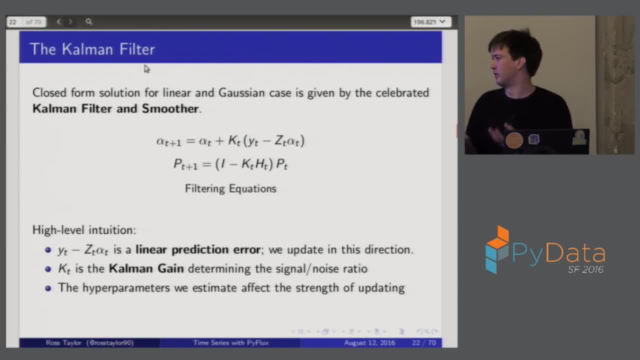 Then you're going to want, according to this equation, you want to up your state prediction to try and get closer, given the new information you have. So you're basically responding in the direction of this prediction error. And the Cameron gain term here is kt and that's going to basically determine how much. 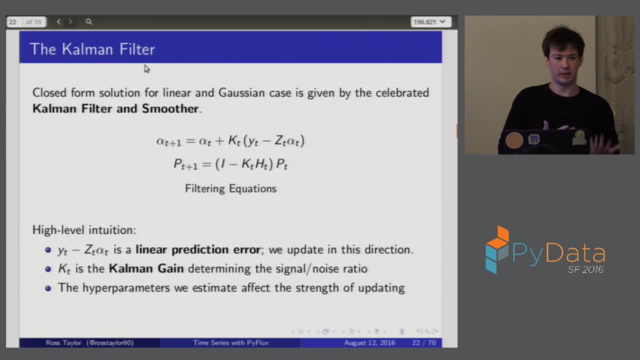 you react to this error, So it's a bit like a learning rate if you come from a Combscay background. It's basically your reaction to this information, And what we actually estimate in this model is hyperparameters which determine the strength. 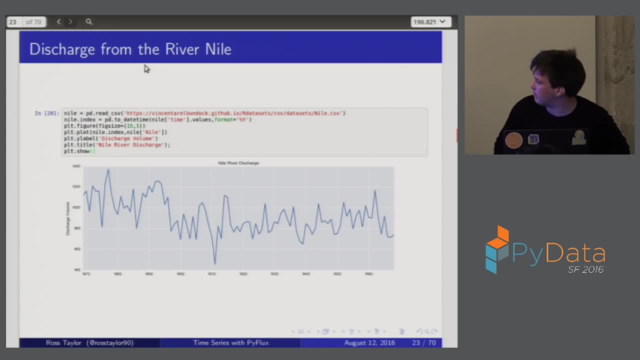 of reaction. So here's a classic example. So discharge from the River Nile. So what does this mean? This is just the water that comes out the delta of the Nile, And so this is a good thing: to apply a simple state space model to. 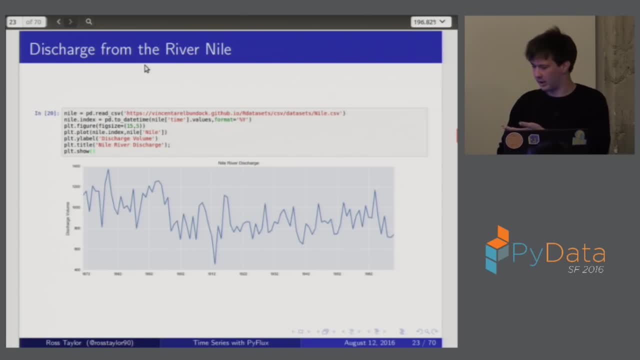 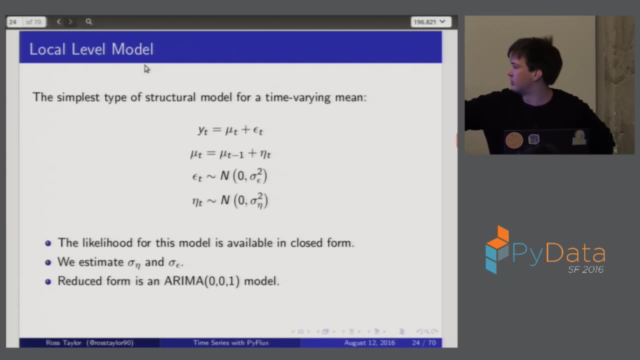 So let's imagine we want to know how the level of water coming out from the Nile has changed over time. So the simplest type of structural model is a local level model. So what's going on here? We have a univariate series and we have it as a function of a time-varying mean which 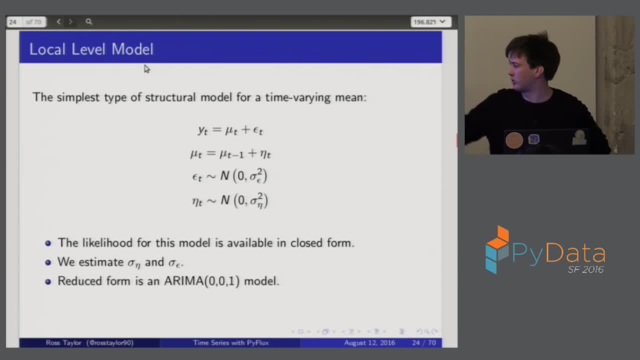 is this mu term And we assume the mu term is a function of a random walk. So that's capturing the variation of a time. If you haven't come across random walks before, just think of like a drunk guy in a desert, Like he's not going to really stay to one location, he's just going to kind of like 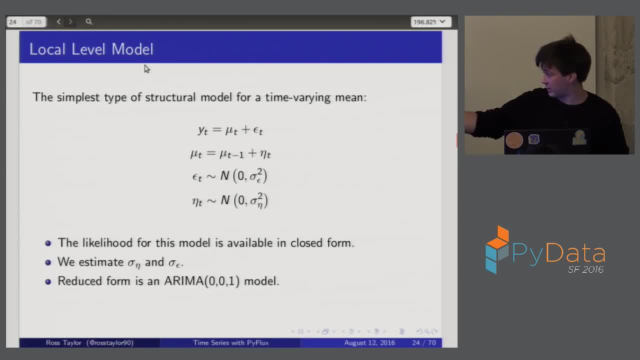 wander around So like. and the important thing is, for the linear case, we have a closed form solution for this, for the Cameron filter, and we're going to estimate these like variance parameters, which again is just the signal-to-noise ratio, if you like. how much would react? 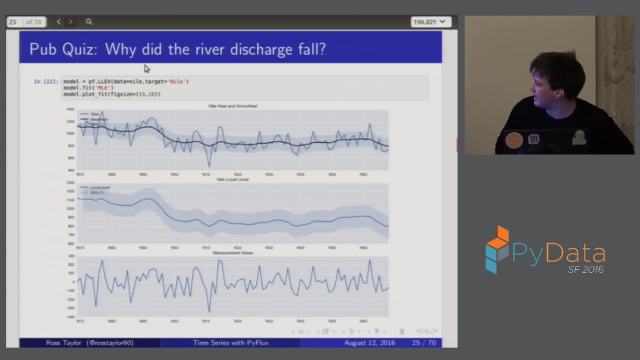 And so this is the smooth estimate and it's very nice. So we see that in the late 1950s, Second century, that's a long time ago- The mean is going down to a lower level And you can see it's smooth. so that's why it's nice and smooth, because we're using 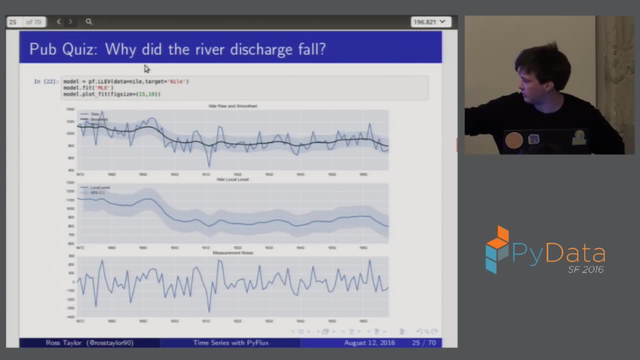 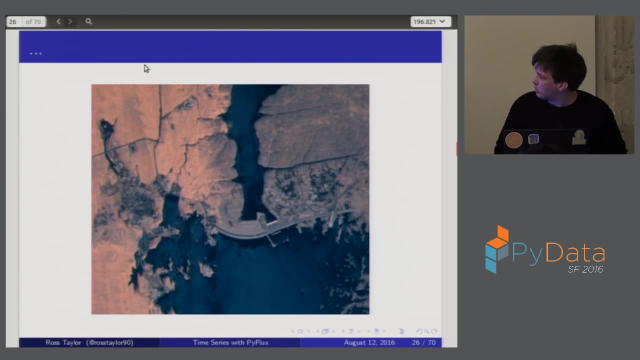 the future data as well, just to do analysis here. So that's the level you can see, it's the value of time and that's the measurement noise at the bottom there. So this is why it actually fell. They built a dam. 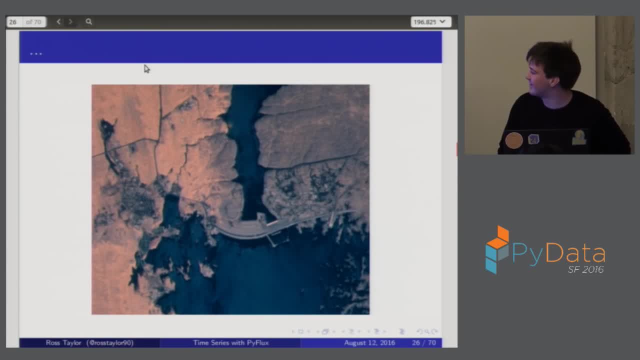 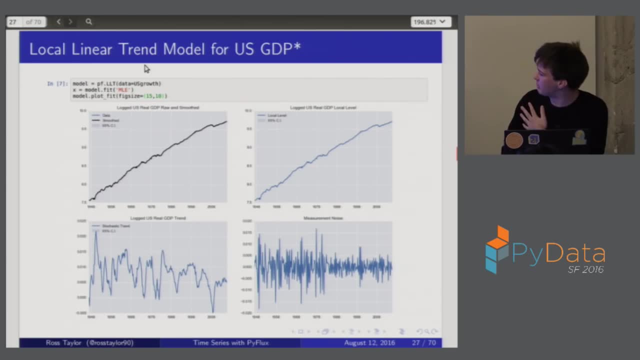 So it's like kind of obvious, right, But it's nice that a simple model like this can capture something like that. And I'm not going to go into detail on this type of model. but stress is the signal extraction point. So rather than say with an arrow model, what we do to remove a trend is, we might like fit. 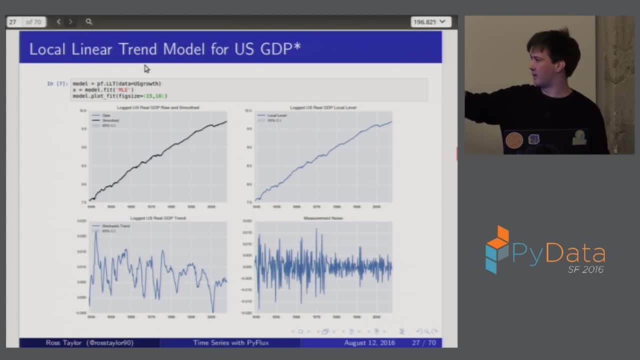 like a linear trend or something. In this type of model we have again a local level, but we assume the trend like varies over time. So this is for US GDP, so it tends to go up and what we can capture in the bottom. 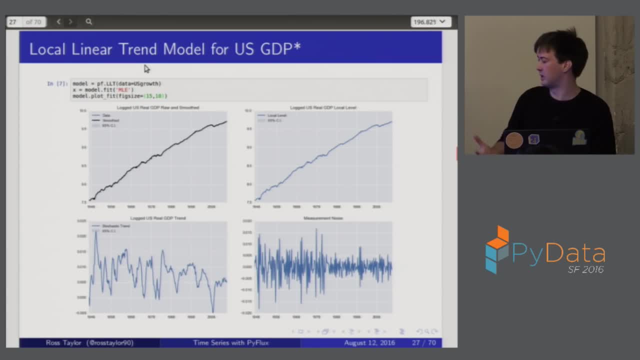 left here is just the underlying growth rate. so this gives an idea of the underlying growth strength of the US economy. So, for example, after 2008,. we're kind of in a like low range. Yeah, I say we. 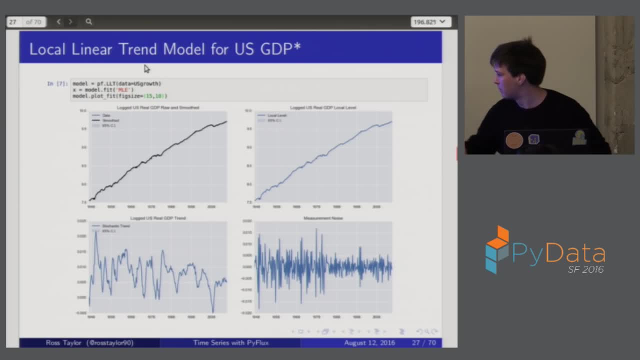 I'm from UK. I'm not going to talk about Brexit. That's a whole load of bloody problems, But the regime here is like- yeah, you can see it's like a lower regime than it was in the past. But, as I've said before, GDP is actually a pretty bad measure, but let's not go into 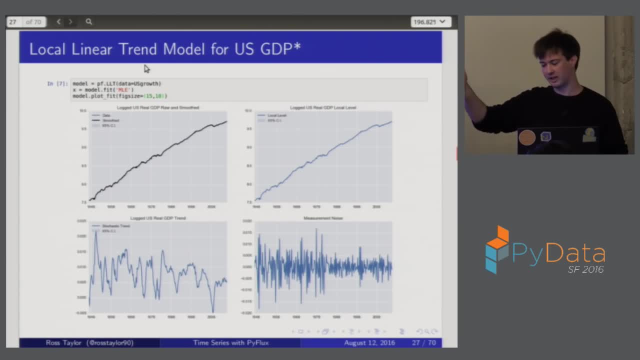 that. But you can see the principle right. We've extracted a trend and, instead of just like capturing it through some lags, we have a really intuitive thing. So you can show this to someone and say, look, this is where we think the trend is and it's. 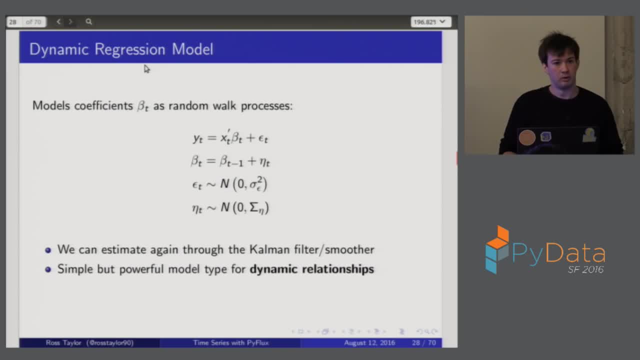 lower. It's very interpretable. What's that? Graphs, whatever? Oh, yeah, The graphs are done. Yeah, It's done using Seaborn, So it's kind of like, yeah, extension to map all that. 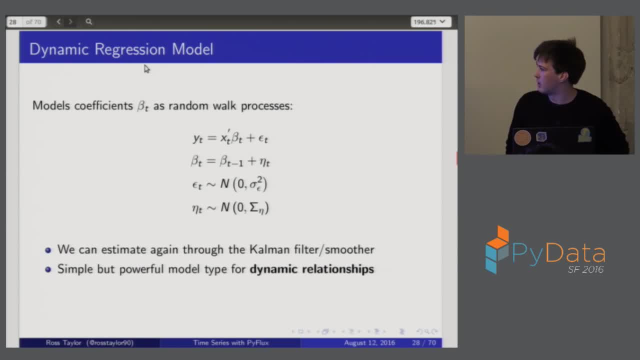 Yeah, So dynamic regression models. So now we're getting a bit of ROM. but imagine we just have a simple problem like a linear regression or something. but we think that the coefficients vary over time. That's a perfectly reasonable thing. we could expect to happen for a lot of data. 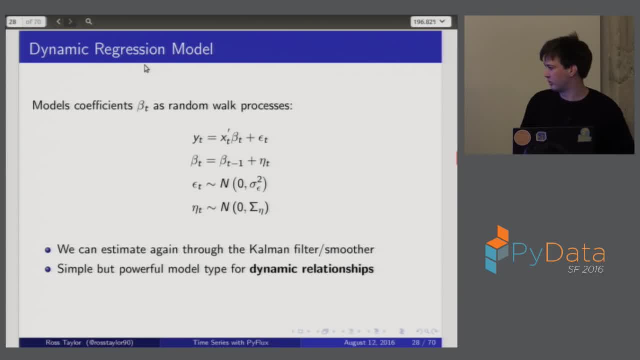 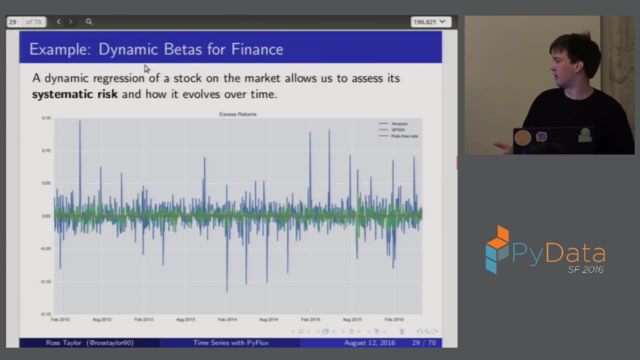 So now it's the coefficients which are following random walks and we're going to model this. So this is simple and powerful for dynamic relationships, And here's a finance example. So in finance, what we're often interested in is trying to find a systematic risk. 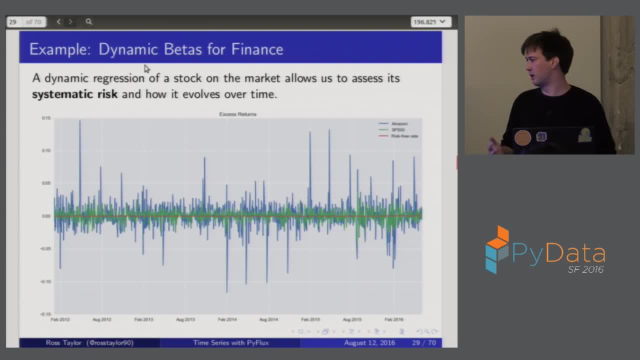 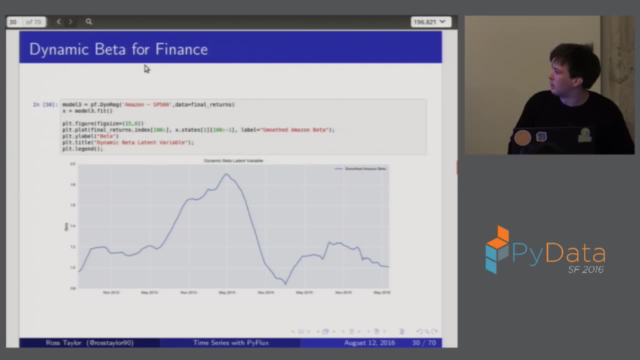 So, for example, if you imagine a stock, We want to know how much of the variation is due to the market And in this case, we want to know how much is like. you know how does it vary over time? That's a systematic risk. 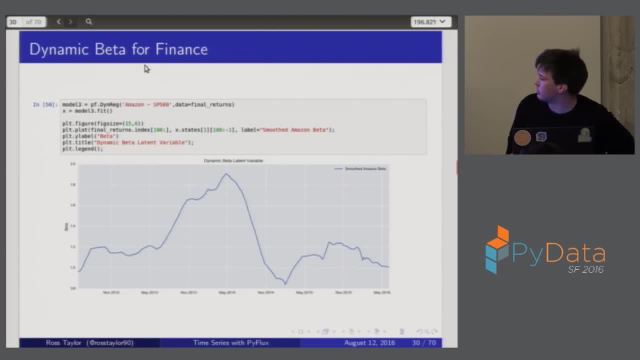 So here's an example here. So I've set up a dynamic regression model and I've specified what I want to regress on, like using Patsy notation, So Amazon on the S&P, which is like the market, And like: here's a smooth estimate. 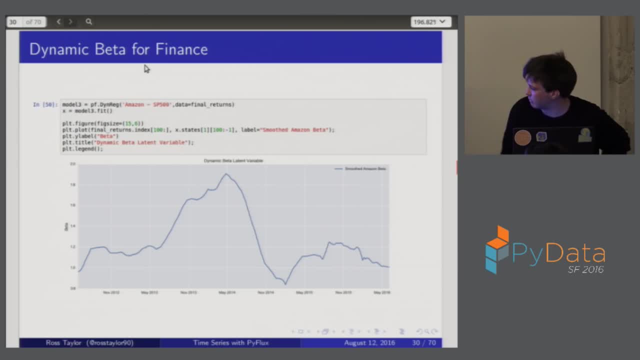 So you could see example 2014,. there's quite a lot of systematic risk, it seems, and it drops down closer to about one In terms of the intuition. if it's above one, then it's reacting heavily with the market. 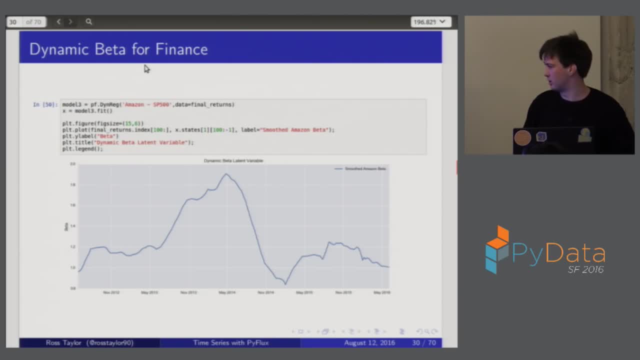 like more than the market. If it's below one, then it's not really that correlated with the market, But there's a problem here. So I'm showing you a smooth estimate Now. if we imagine actually like using like betas and like finance, then we're probably 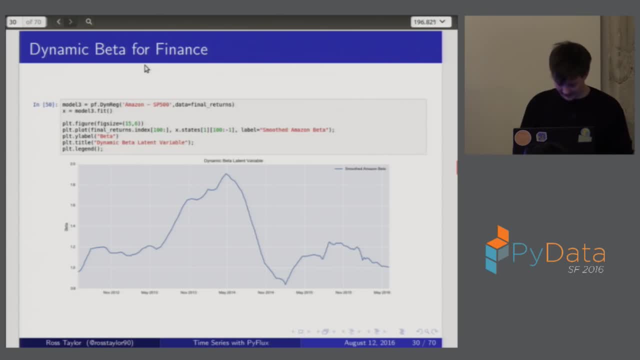 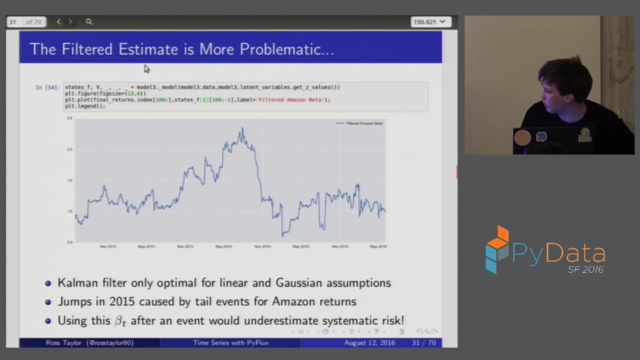 going to be interested more in the filtered thing, like: what do we think now? And the filtered thing has some problems. So do you see in like 2015,, these massive jumps down. So it goes from about one to almost 0.5.. 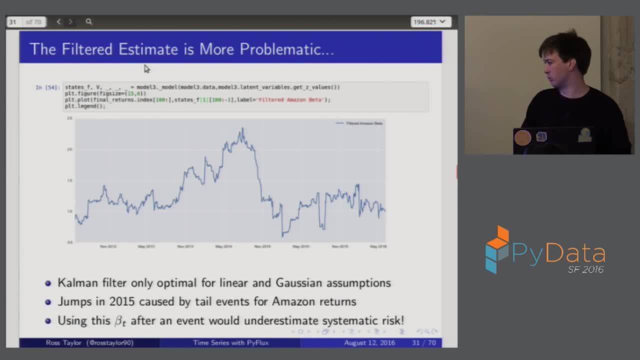 These are big jumps, So this is a limitation of the model we're using, which the Cameron filter is only optimal for linear and Gaussian assumptions. So the jumps in 2015 are caused by tail events, which I'll show you on the next slide. 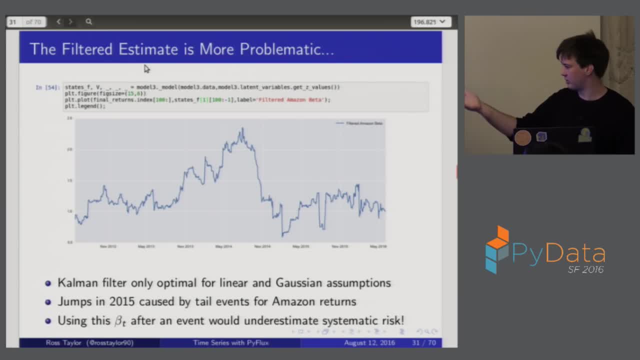 So if we're using a filtered estimate and using these assumptions, then it's not particularly useful, Like if we use the beta after a jump, then we're going to potentially severely underestimate systematic risk, which is not good at all. And this is showing the components. 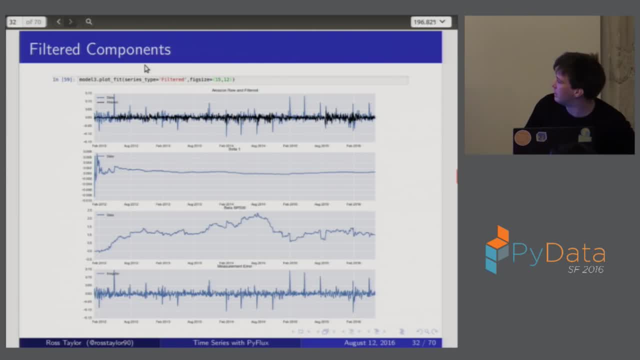 So if you look at the top graph, if you look at like 2015,, you see there's a massive spike. So for Amazon they've had, like, for example, big spikes And the reason why it goes down the beta is because there weren't corresponding spikes. 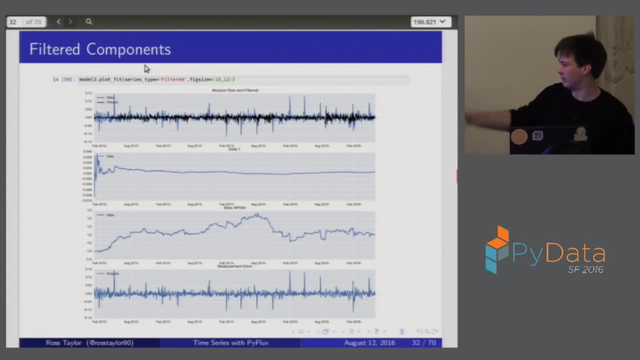 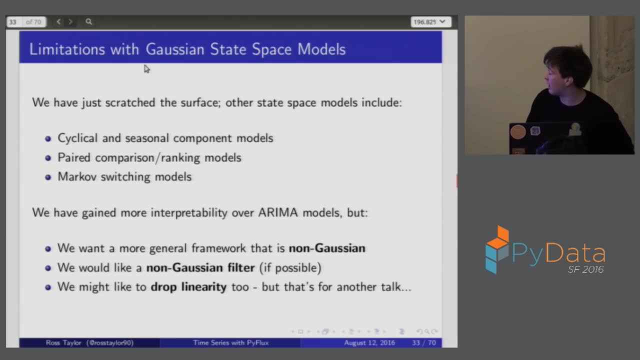 for the S&B 500.. So these were idiosyncratic events for Amazon And that's why you get these weird jumps, which aren't very desirable. So limitations. Now I've only just scratched the surface. So state-based models capture so many cool things as we could have- cyclical and seasonal. 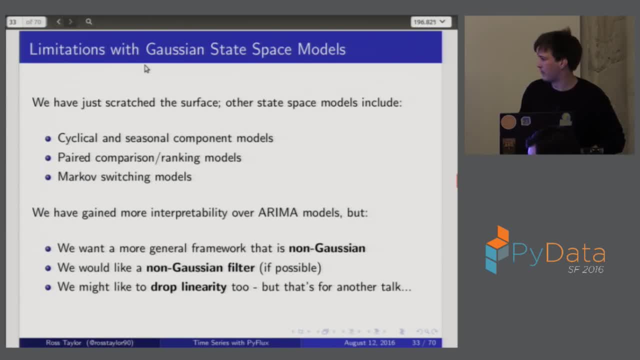 components, ranking models, mark-off, switching models And like. while we've gained more interpretability over our own time, we've also been able to do a lot of things. So let's look at some of the Arama models. Like there's some problems here. 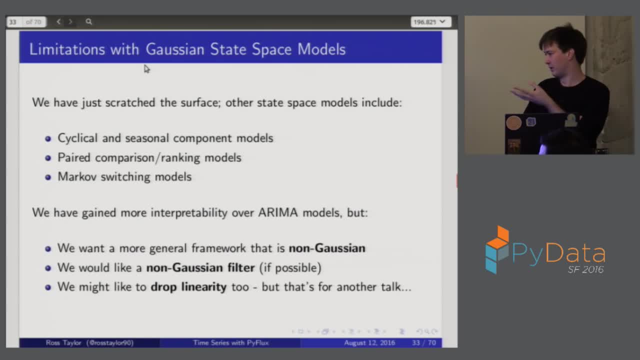 We want something that's non-Gaussian. We've just seen something where a Gaussian assumption- implicitly, if you like- isn't really working for us. Ideally as well, we'd like a non-Gaussian filter. Like there are smoothies available, but a filter is kind of useful for, like, a lot of. 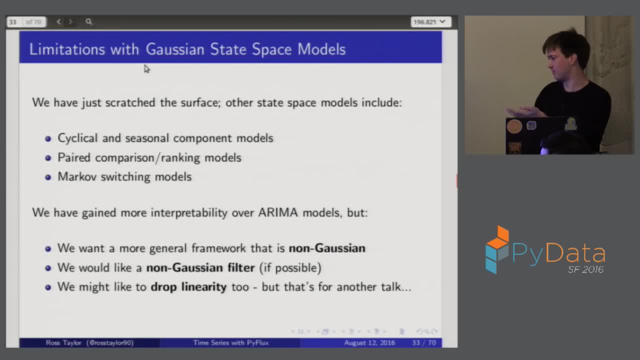 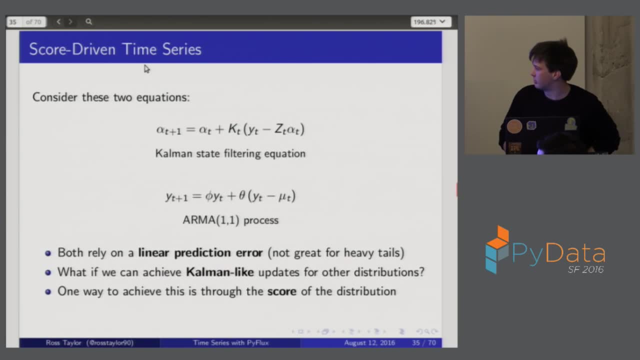 practical problems, And we might also like to drop linearity, but that's for another talk. So score-driven time series. So this is like a new type of model that I want to introduce today. So let's revisit the Cameron filter and also the Arama. 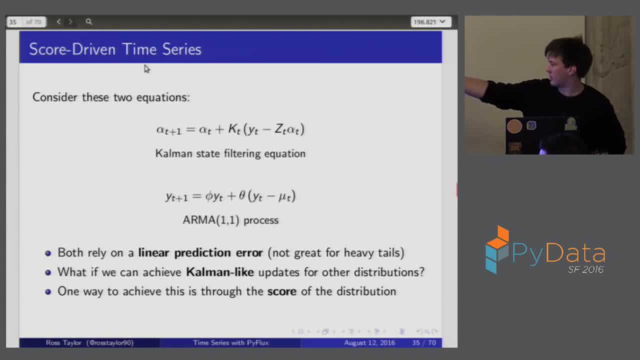 So let's have a look at this equation here. So the state equation is evolving according to a linear prediction error, And that's why you're getting these weird events. with the beta thing you saw a few slides ago, It's reacting linearly to these shocks. 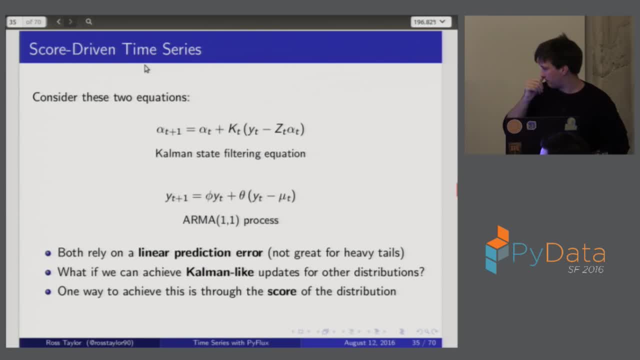 And actually if you have a massive tail event, it's going to react quite a lot. And also the Arama you know, for example, has a similar thing here. This particular process- you see the yt minus mu t, similar to the yt minus zt alpha t. 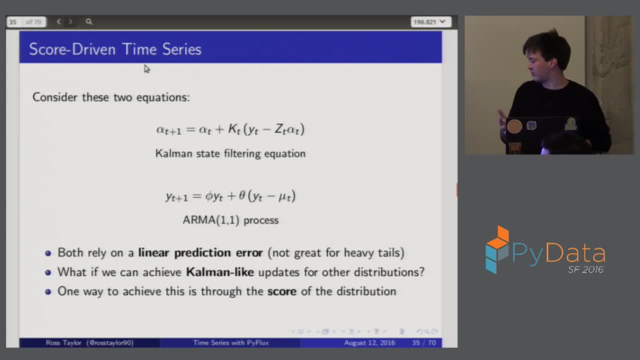 This linear prediction error is causing problems. So one of the motivations for score-driven models, which I'll introduce in a bit, is that we want to achieve something that's Cameron-like, Because the Cameron filter is pretty elegant, useful and quick. 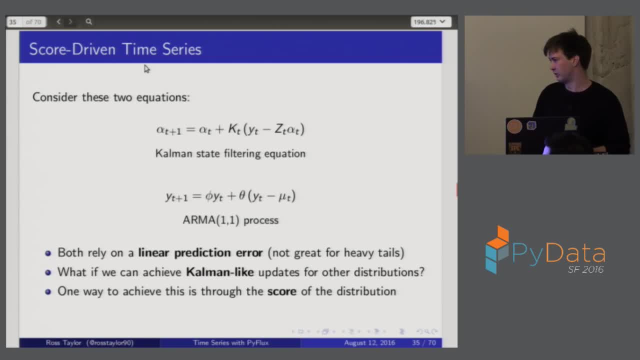 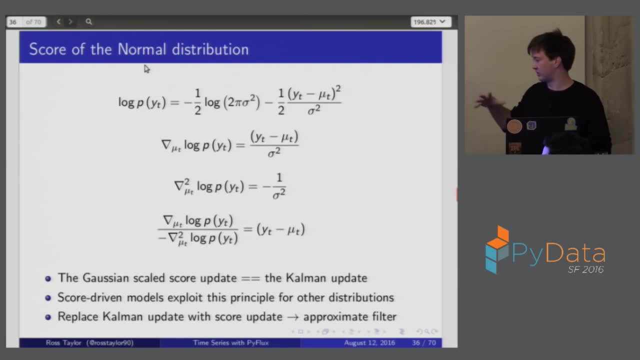 But we want it to have something like the Cameron filter for other distributions, And one way to achieve this is through the score of the distribution. So what is the score? So you don't have to go through all the math. It's actually pretty simple if you go through it. 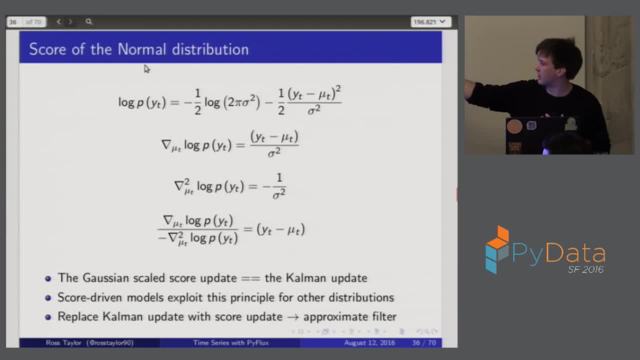 But let me just show the intuition here. So basically, this thing at the top here, this is the log density for like a normal distribution And basically if we just take derivatives and we get like something like a Newton-like, you know something like that. 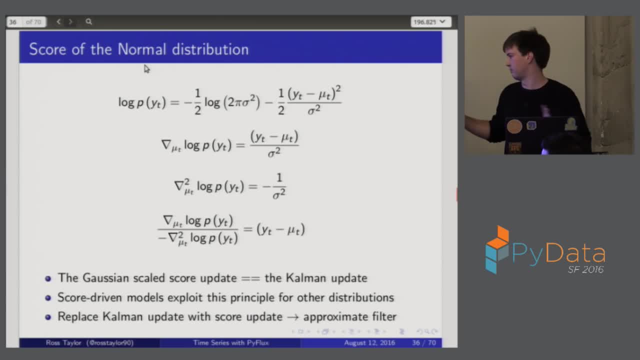 Like a Newton-like update. If you don't come across like Newton-based methods, don't worry, But basically the point is here for the normal distribution, you see, this linear prediction error comes out again. That's like the way to update the parameter for this particular point in time. 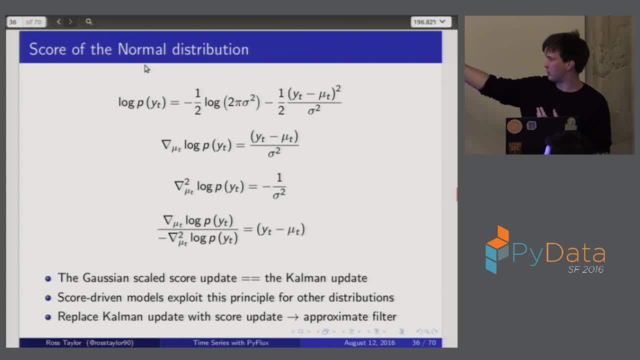 So basically, the idea is, given that the score of the normal distribution, which is basically derivatives, is Cameron-like, why don't we exploit this principle for other distributions? So again, for example, we can look at Poisson distribution And again we take derivatives and we get like an update term. 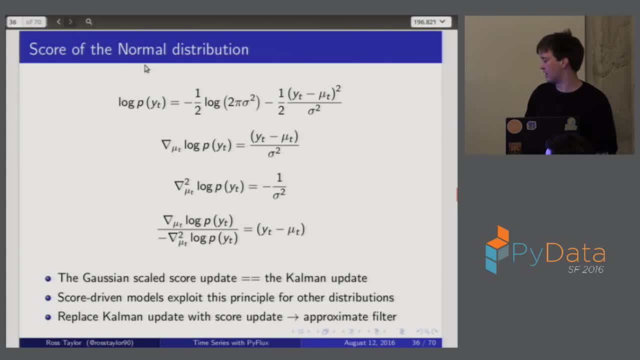 Which we can use, which is like a bit like the Cameron filter. So this is the basic idea. We want an approximate filter for other distributions. So that's a good question. So exponential family models: it tends to work best with them. 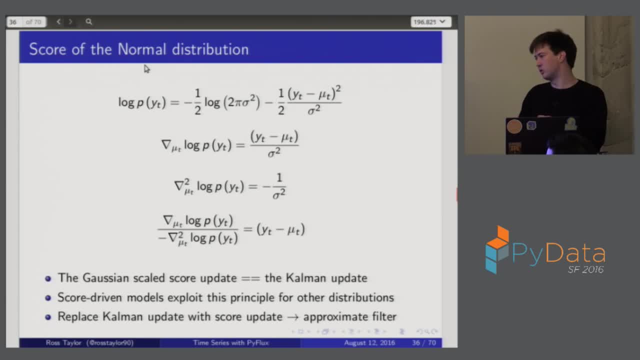 But you can use other things which aren't in the exponential family. But you're right, Once you get, like you know, things which are like differentiable and things like that or the second derivatives are a bit messy, it kind of loses its appeal a bit. 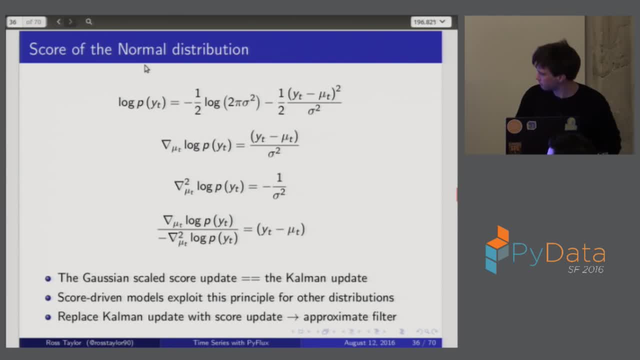 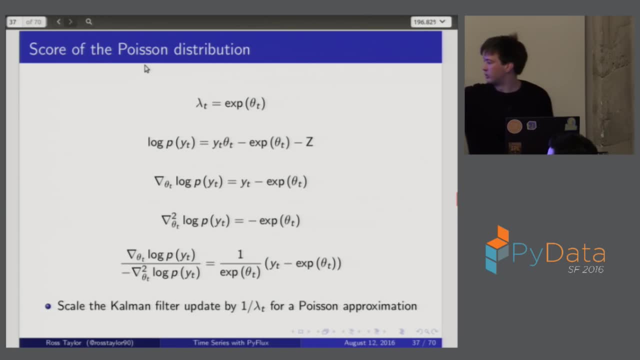 But you can technically- yeah, still- do it for non-exponential family models, Yeah. So what do you mean by the score specifically, The score specifically. So on this guy here, for example, the score is just going to be the gradient in Willem. 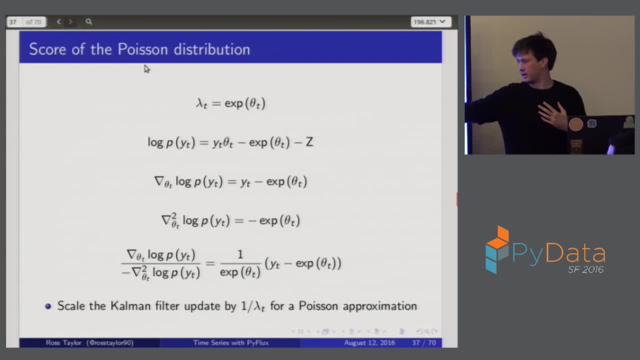 terms, But in these models we can actually scale it, if we like, by the Hessian-based term as well, to get something which is a bit more It takes into account, like the quadrature, So it's a bit like a Taylor approximation. 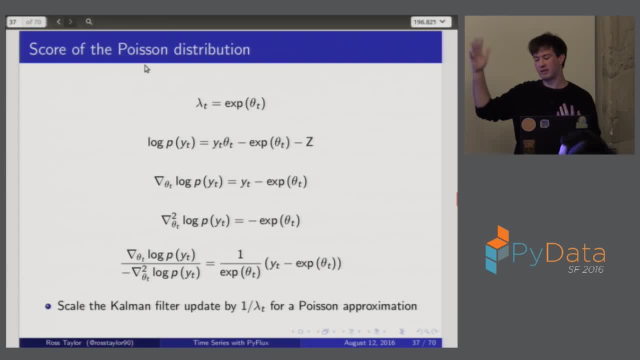 But a score, specifically, is just going to be the derivative. So you could have like a simple score-based model which just uses the gradient And it represents something a bit like: you know stochastic gradient, You know stochastic gradient, descent in a way. 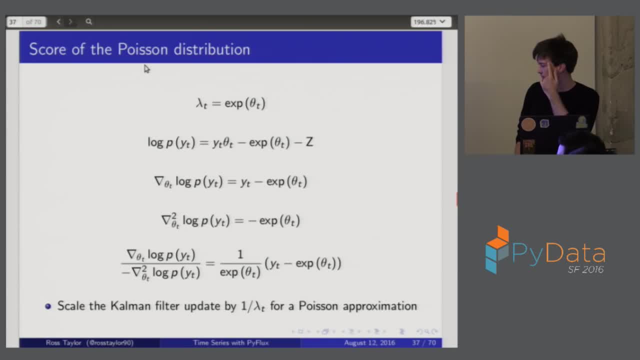 So you can basically use any degree of you know complexity with those derivatives. So again, don't have to go through this. but basically for the Poisson thing, we have something here And we basically have a scaling term here. So that gives us like an approximate filter for the Poisson distribution. 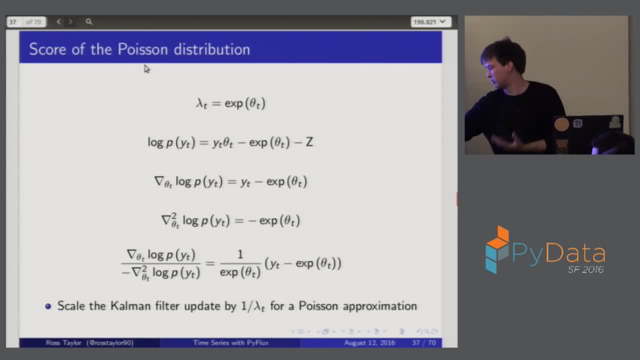 So we have an error term: Exponential theta. here is basically where you think that the Poisson rate is going to be And we have a scaling term here, exponential. But you don't have to worry about not understanding this fully yet, But the Poisson is going to be here. 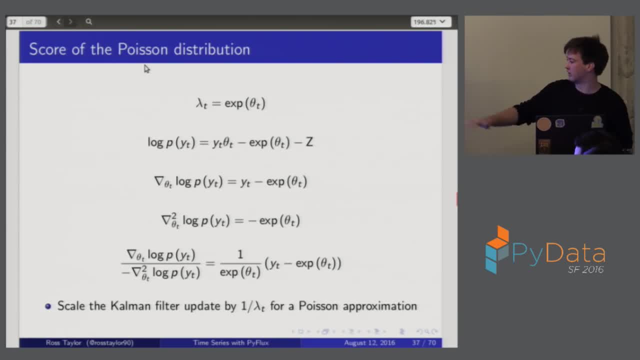 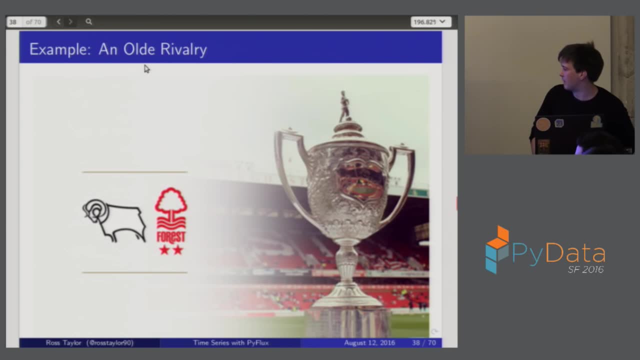 Yeah, Yeah. So the point is, we can, you know, take derivatives and get something approximate. So let me give you an example. So my dad's side of the family are from Nottingham, which is a town in England, And they all support Nottingham Forest. 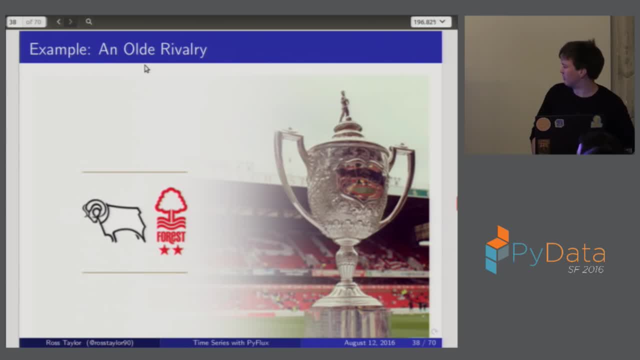 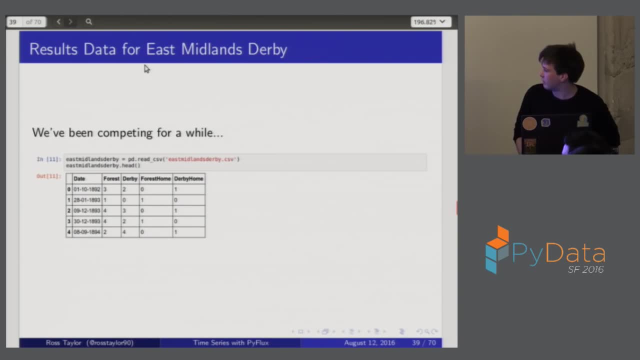 And they compete with a side I don't really want to mention or promote the name of, called Derby FC And they have a rivalry And they've gone back like basically since 1896.. So I've just got some data here on the scores for these two teams. 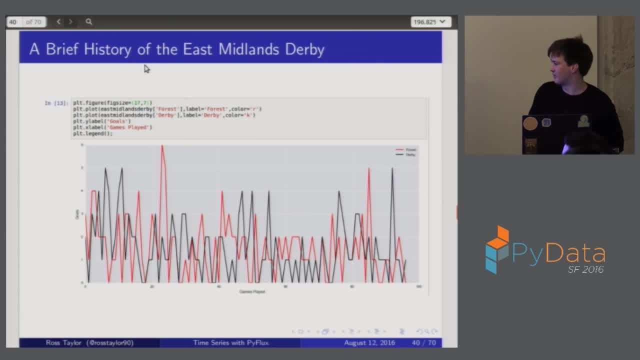 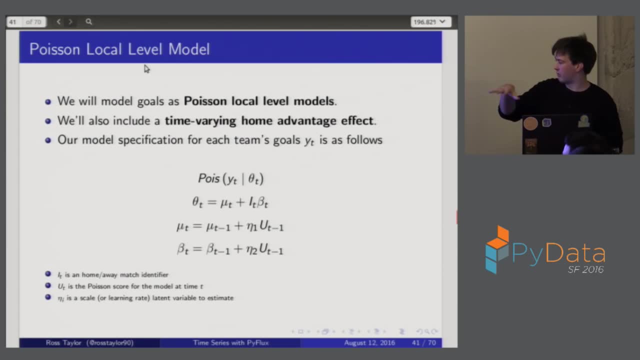 And you can see this is what count data tends to look like. So it's quite hard to identify Like trends and things by just eyeballing this stuff. But this is classic count data. So I showed you like the river example for like a Gaussian local level model. 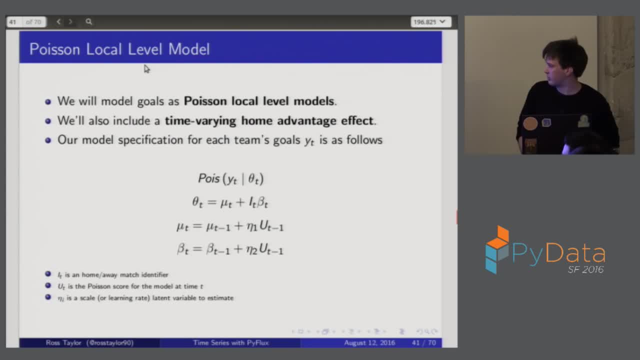 Let's do a Poisson local level model just using the score. So what I'm going to do here is I've got a Poisson assumption for each team's goals And I assume the rate is going to be a function of a local level. 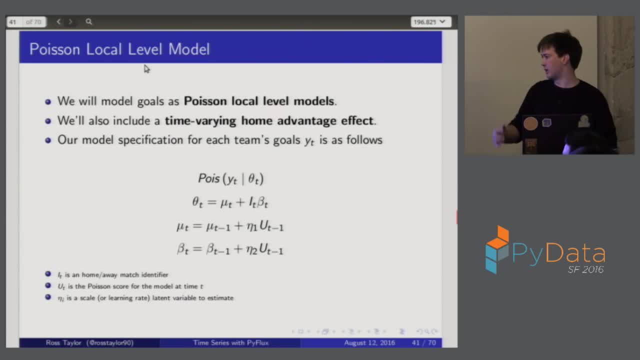 So we're assuming that the you know, perhaps the goal scoring rate of each team varies over time And also a time varying home advantage effect, Because home advantage tends to be a big thing in sports, And here's an example. So I've set up a gas regression. 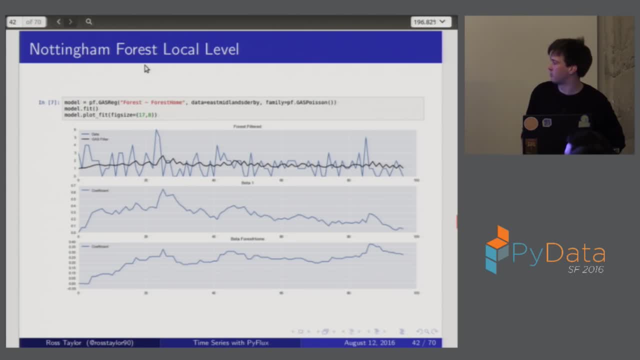 And I've regressed Notting Forest's goals on, say, a home advantage parameter, Plugged in the data And I've chosen the family I want. So I've used a Poisson assumption And you can see the variation over time. 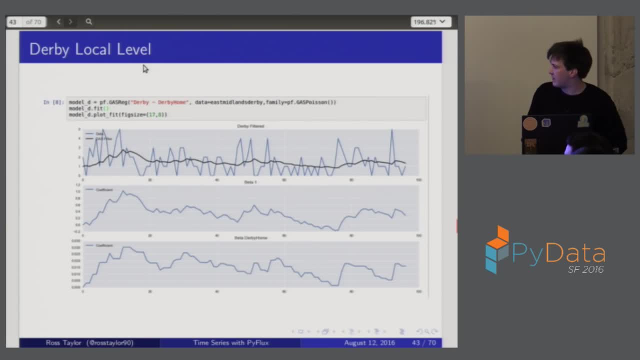 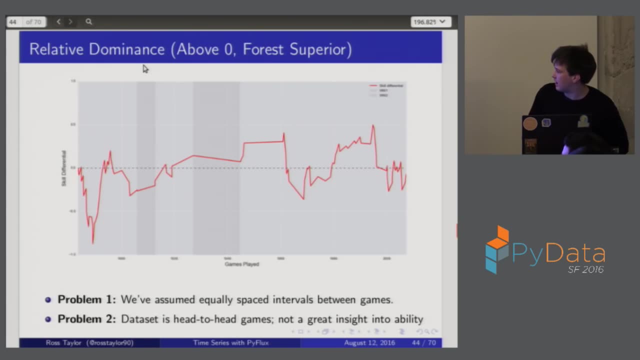 You can do the same thing with Derby. And then what I've done is basically, if you combine these two results, you can get a very crude relative dominance measure over time. And so you can see I've actually- that's not games played, That's the year. 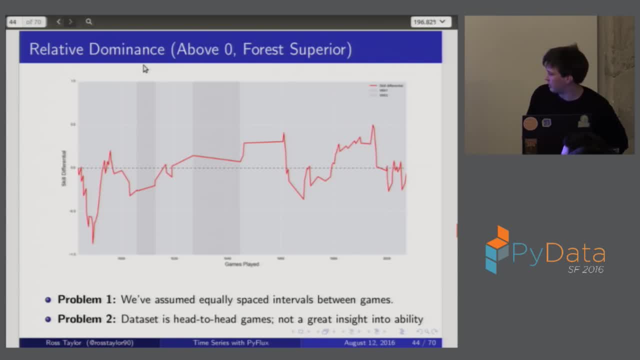 And then I've got a very crude relative dominance measure over time, And so you can see- actually that's not games played, That's the year, And I'm going to talk about it in a bit- If they're above zero, then based on these head-to-head results, we think Forest is superior. 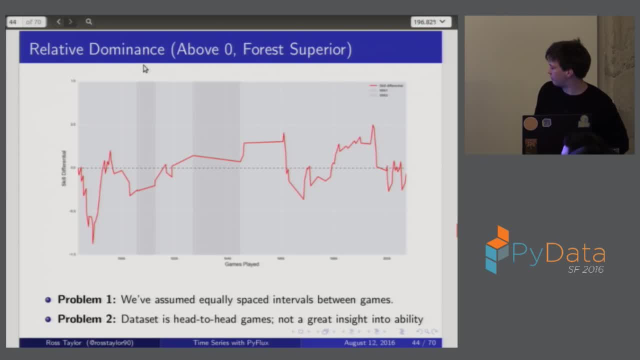 If we think below zero, then we think Derby is superior. But this is very crude. We've assumed equally spaced intervals between games which you see. these you can't really see on this screen, But you know, there's a small thing called World War I and World War II, which stopped. 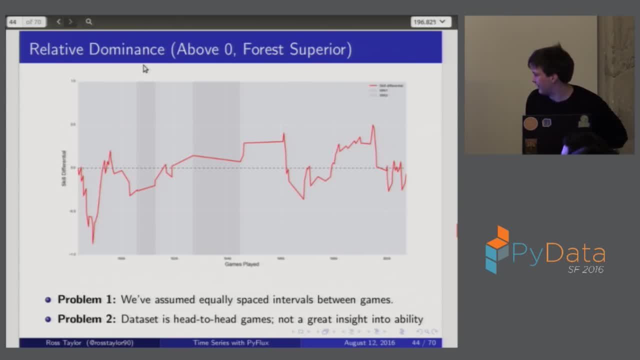 football, unfortunately, or soccer, sorry, And also it's head-to-head games, So it's only the games between these two teams. That's not a great source. You want to see, you know, how good these teams actually are. 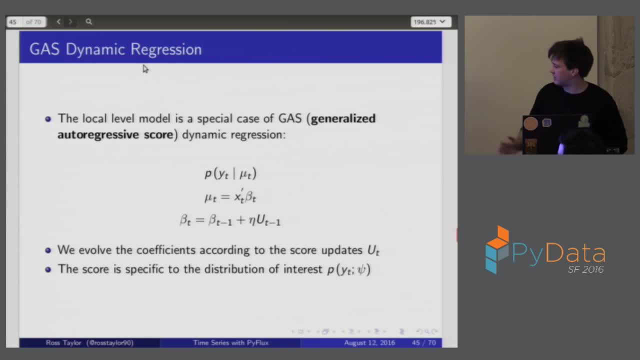 But you know that's a good start And these types of models they fit into like a more general class, just gas regression models. So again it's like the dynamic regression models I showed before, but now we're using 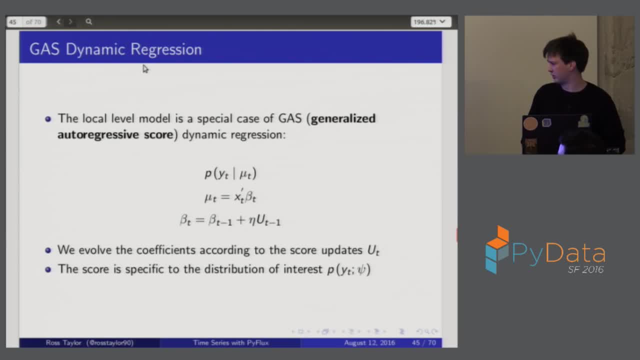 a score term rather than like a Kalman term to update these coefficients, But it's basically something like a random walk again. right, If a beta is a function of its own self plus the score-driven term. So let's go back to that finance example. 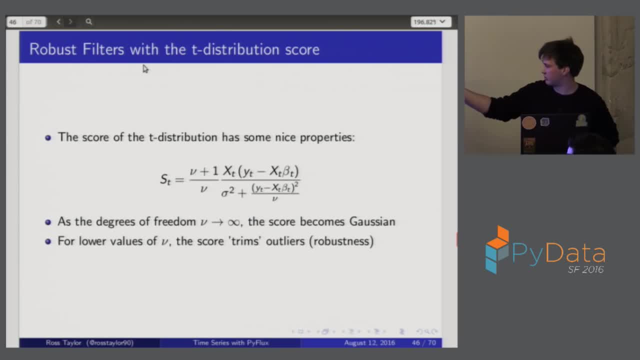 Don't worry about trying to understand every detail of the term, but the score for a t-distribution has nice properties. Basically, a t-distribution has a degrees of freedom parameter. If it's really large, the t-distribution is just Gaussian. 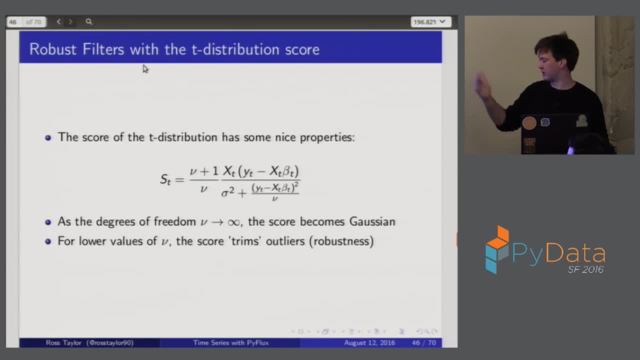 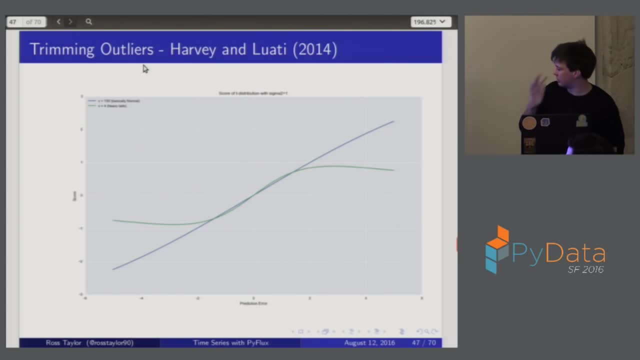 But if it's low, then what you see with this score distribution, as I'll show in the next slide. so actually it's very nice because it trims out lies, so it gives you robustness And this graph is quite useful in this respect. 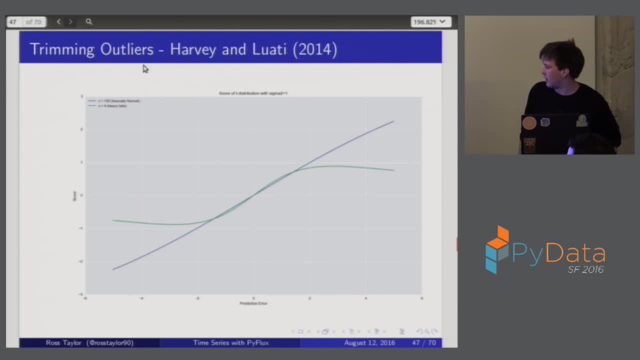 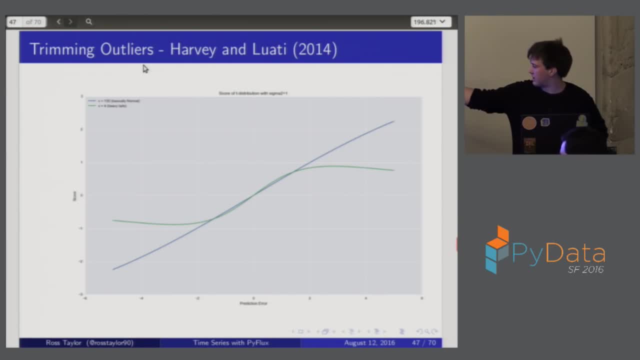 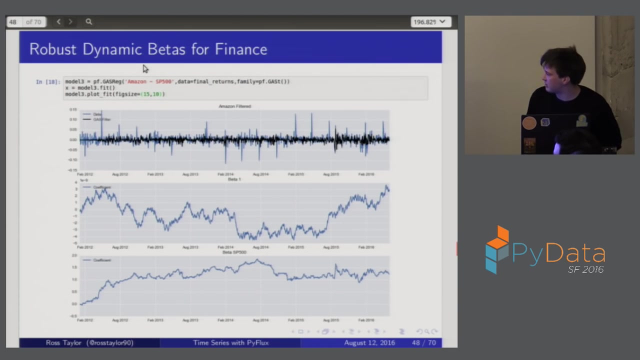 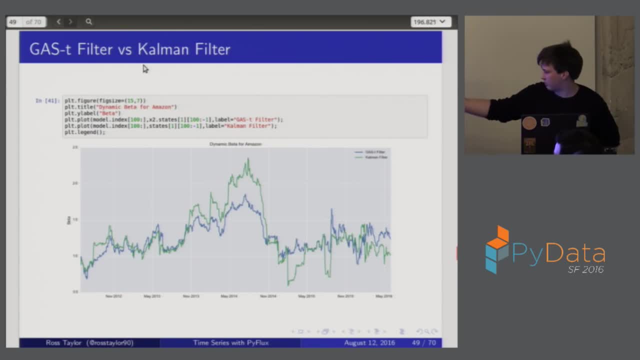 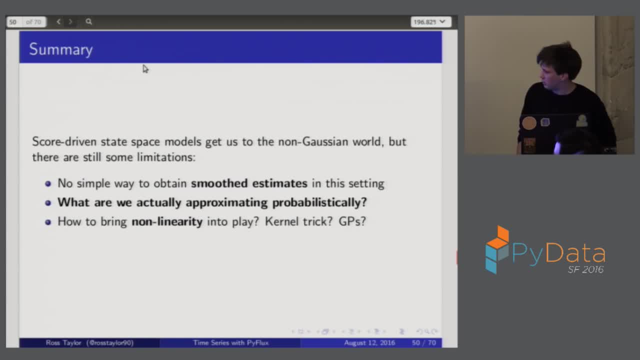 So that's an attraction of that kind of model. So, summary: These types of models get us to the non-Gaussian world. but we have some limitations. There's no simple way to obtain smooth estimates in this setting. You can kind of fudge it a bit, but it hasn't really worked out yet. 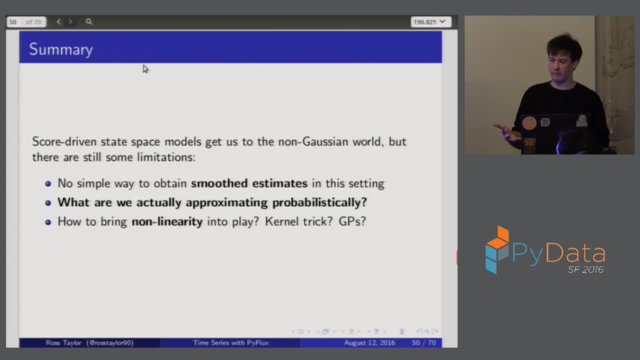 A bigger problem is like: okay, so we're getting something like the Cameron filter, very nice, but what does it actually approximate? So, okay, it looks something like a state-space model, but not quite, So I think that's problematic. 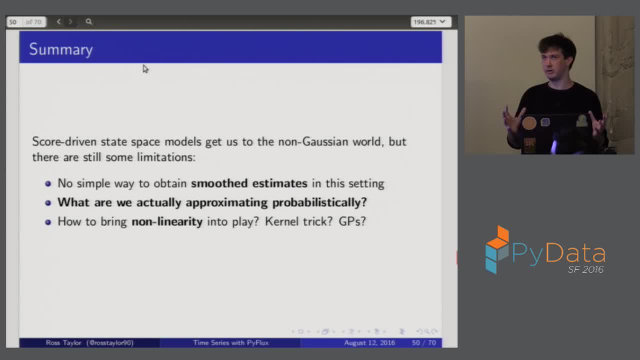 Ideally, when you're doing approximation techniques, you want something theoretical which tells you the degree of approximation. So you might come across things like KL divergence and things like that, which is a direct metric and gives you a lower bound in the approximation. 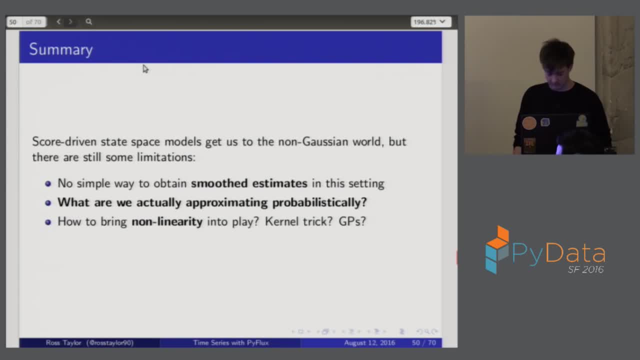 There is something like that with these models, but it's not quite worked out and I think that's problematic, to be honest. And then non-linearity. So we all care about non-linearity these days, So I mean you could have 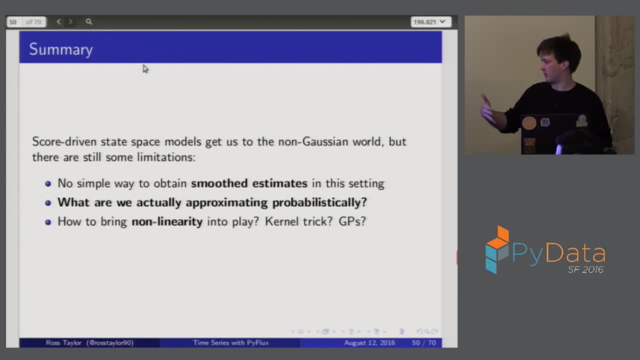 I don't know alternative model type, but there's good ways perhaps potentially to try and get non-linearity within this class of models. So just exploiting things like the kernel trick, which is very useful Also, just like putting in Gaussian process-based terms as well. 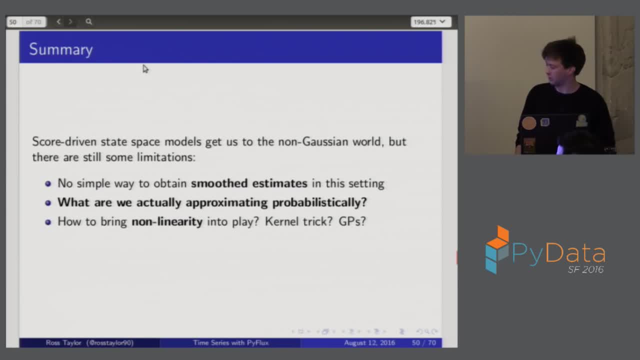 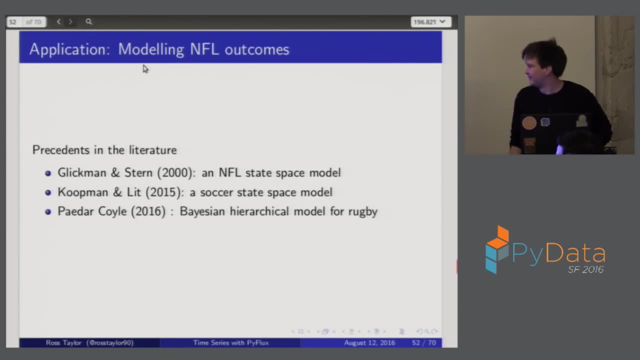 Look those up, even if you haven't had experience with them, because they're quite interesting. Okay, so let's do something fun. Well, fun is fun, right, Come on. We have some precedents in the literature, So a lot of people actually model. 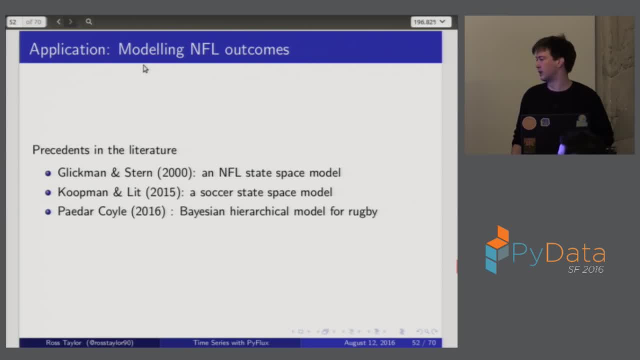 model sports and it's now very popular with sports analytics and you can even see models on 538 and stuff for sports. What I'm interested in here is kind of like looking in this state-space framework- the top two and also the guy here- 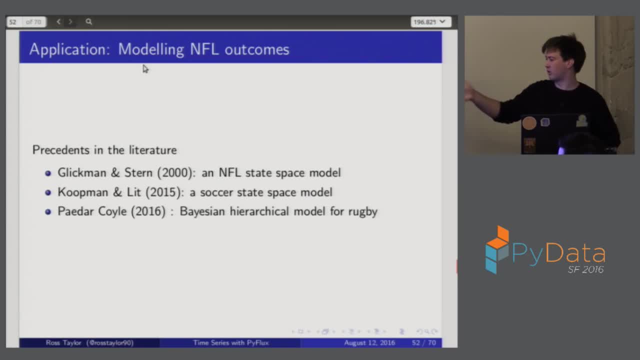 So the top two ones for NFL and soccer, and what they're basically interested in is trying to model abilities of teams over time, how they change over time. And the third one here is also interesting. Hierarchical models are very popular because if you don't have a lot of data in sports 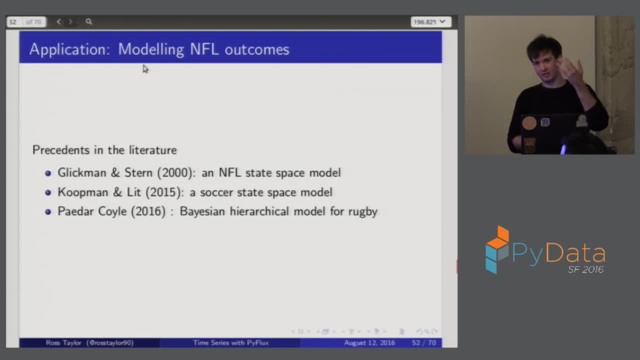 and you just use something like maximum likelihood, then you're going to dramatically overestimate or underestimate ability. It tends to be a bit rough. So what hierarchical models do is they basically pool information. So you can check those out as well, But I'm going to focus on state-space models. 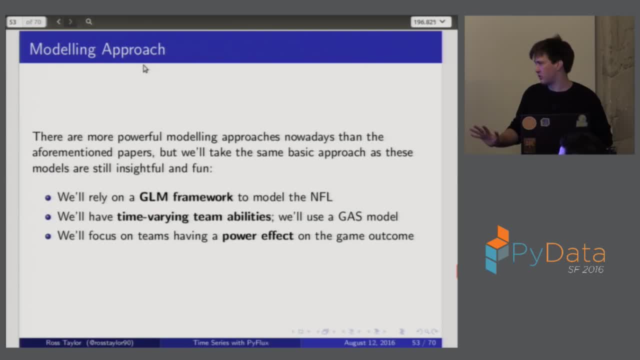 for this framework. There are actually more powerful approaches. these days I can't really touch upon that that much, but we'll take the same basic approach, because this is a great way to start thinking about these problems and it's still insightful and fun. 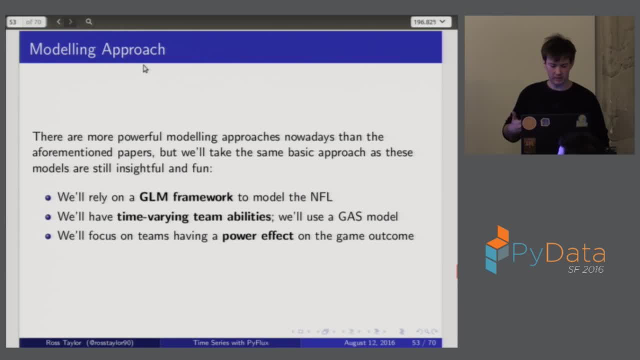 So we're going to use a Glim based framework. So we're going to talk in terms of these, like probability distribution, if we talked about, like Prussell and Norwood et cetera, We'll have time-varying abilities. 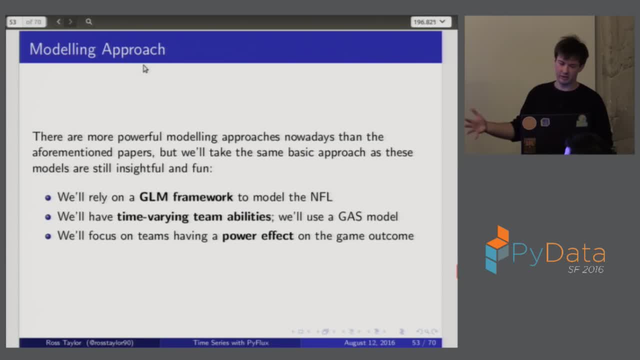 And we're going to focus on teams having a power effect on the game outcome. What a power effect means is basically the team enters like a formula, like a formula for, say, points or goals. Basically it's like a coefficient. So, for example, if it's a soccer game, 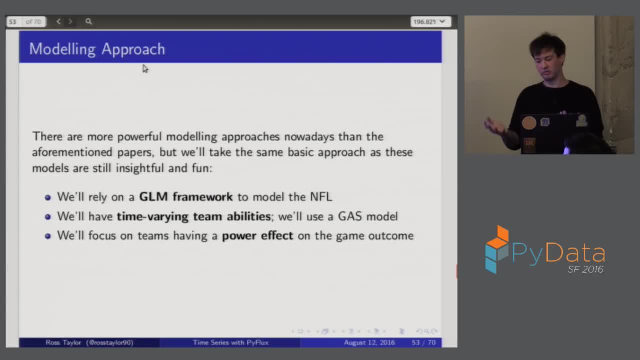 and it's like Leicester versus Hull. we have a coefficient for these different teams and it comes, if they happen to be in that match, So it pops up and they have a power effect. For example, if they have high power, then you're going to get lots of goals. 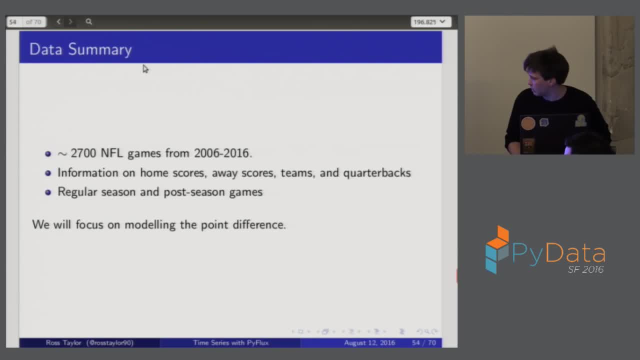 or if they have low power, the opposite. So data: I've just taken some basic data, so about 3,000 NFL games from 2006 to 2016.. We have information on the home scores, away scores, teams and quarterbacks. 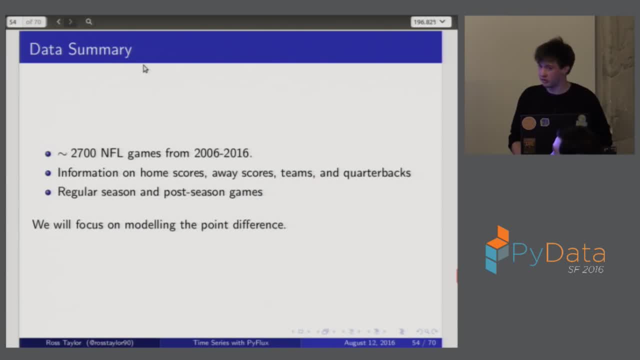 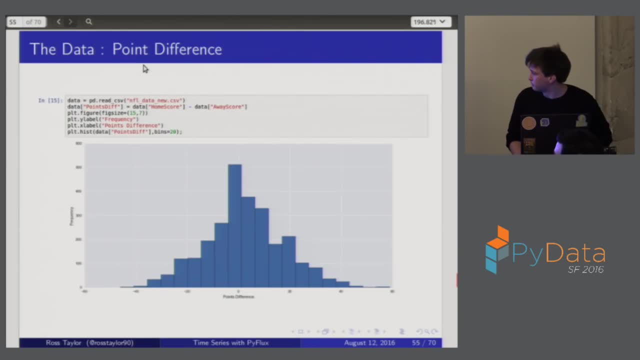 And we have regular season and postseason games. I'm not using preseason games- You should think about why I'm not- And we'll focus on modeling the point difference. So this is what the point difference looks like. So a lot of people just look at this and say: 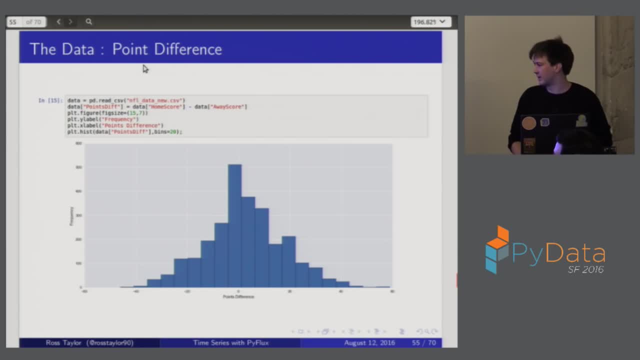 okay. well, it's not quite normal, but we could do something like that And that might be an okay assumption. So if you've read, like you know, Gellman's book on patient data analysis, they use a normal assumption. 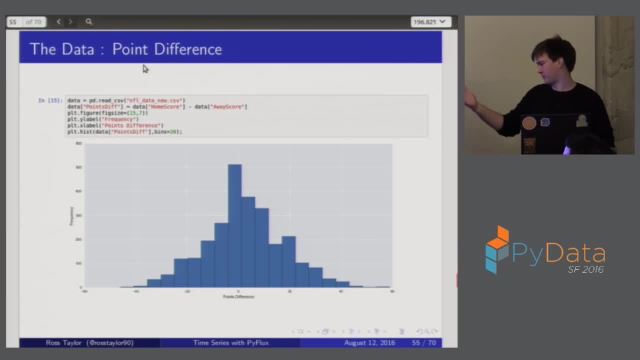 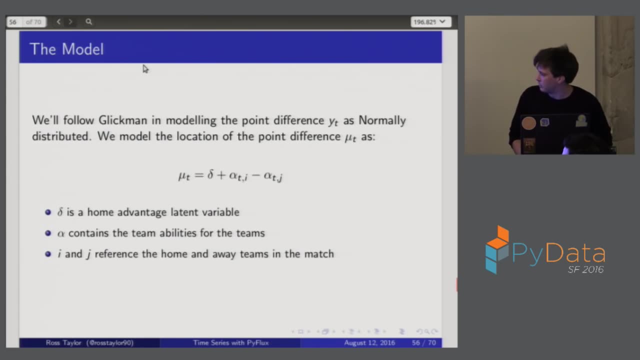 Glickman, the guy I mentioned two slides ago. they use a normal assumption. So you can actually use more complex things like which account for skewness and stuff. but let's just go for a normal distribution. We'll assume it's normally distributed. 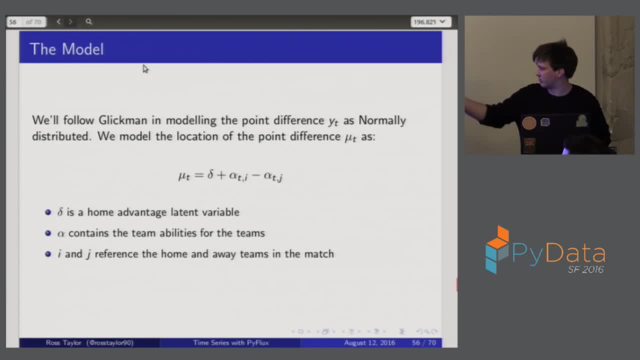 And this is the model we're going to go for. So we assume the point difference. we're going to model it by this location parameter, mu, We assume it's a function of a home advantage effect and these power terms. So imagine time two. this is a match or something. 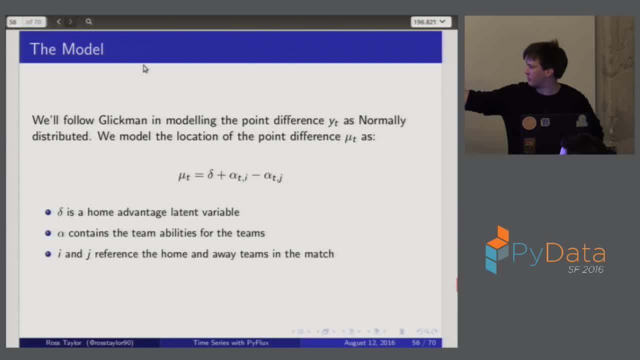 I think the indexing is a bit wrong. I don't know if it's wrong here, but whatever. So we have a home team, alpha ti, and an away team, alpha tj, And the power is going to affect where we think the expected points are for these teams. 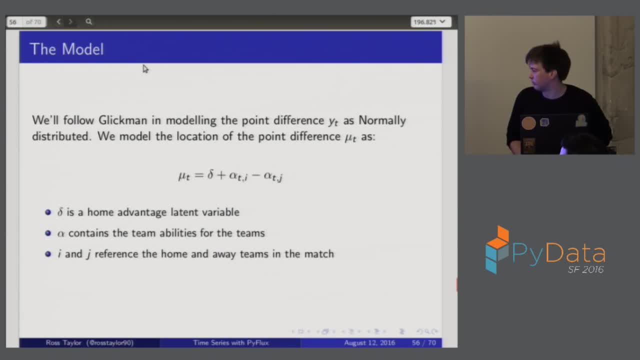 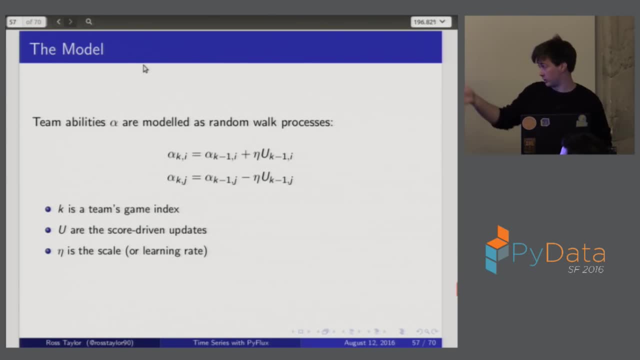 Does that make sense? Cool, And we're going to model these team abilities as random walk processes, But we're using the gas term here and it's going to be for the normal distribution to try and drive these dynamic updates. So you can see, i and j again are home and away teams. 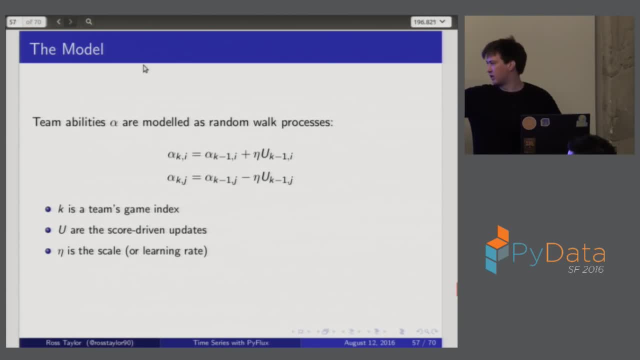 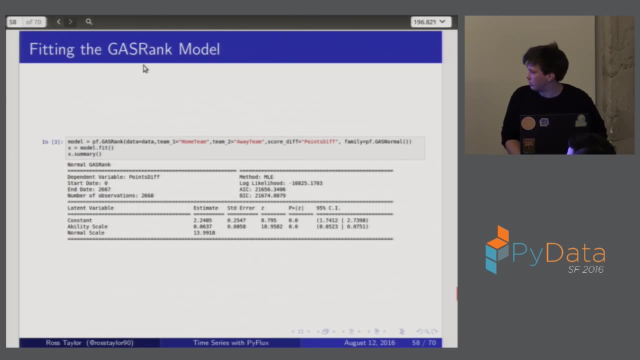 And again they're following random walks. The sign is negative here because one of the teams is the away team and they're obviously going to have a different sign effect on the point difference. So I've just included this recently, just for fun. 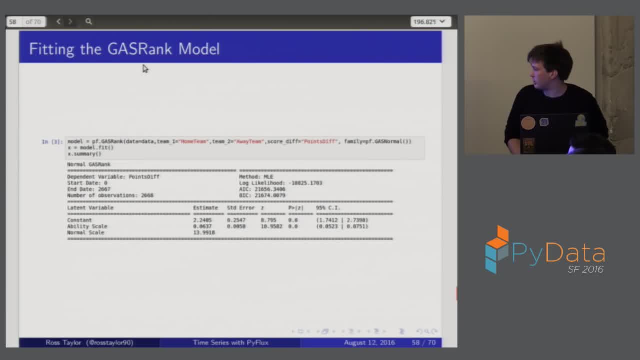 So you basically define the data, Define the columns which are specifying the home team and away team strings, Define what's the point, difference or score difference. So here NFL it's like a points diff. It could be something like goals diff, if you're. 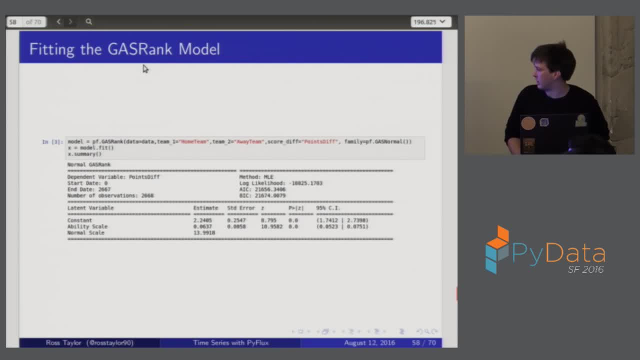 doing soccer or something And then define the family you're making the assumption about. So we just assumed a normal here And we're doing sports like soccer. for this very basic model, We might want to do something like a skellum, which. 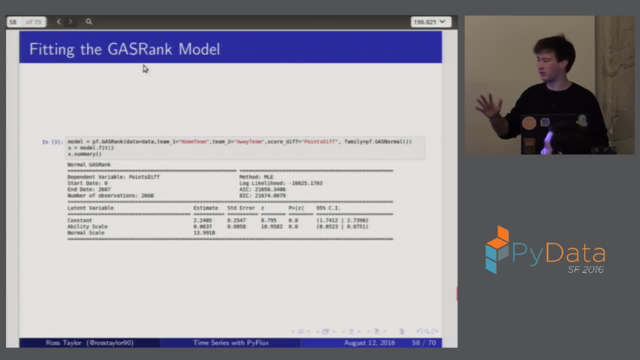 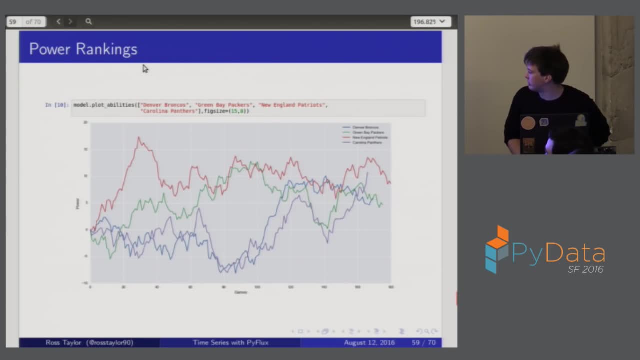 is just like a distribution, the difference between two or something. Basically, the point I want to get is there's a difference in some things you can make here. So here's some output. So I don't know what teams you guys support. 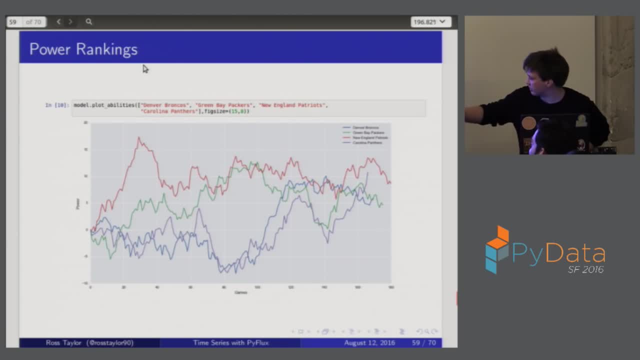 but I've got some graphs here And you can see the games they've played since 2006 and how they've evolved over time. So we have here the Patriots, who are basically a dynasty. for the past 10 years They've gone through legitimate or illegitimate means. 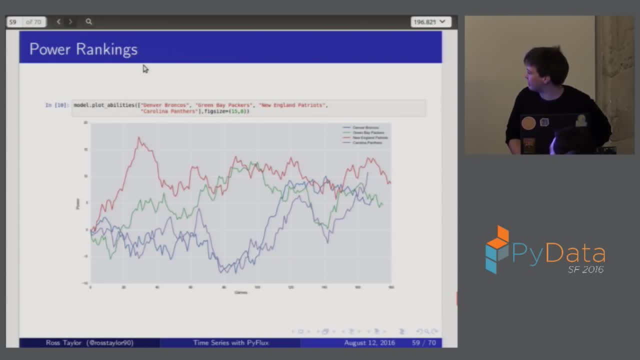 I don't know, Sorry. And we have a team like the Panthers, who have become very prominent in recent years because they're shooting up Denver Broncos- they've gone up recently- And we have Green Bay Packers who are kind of goodish. 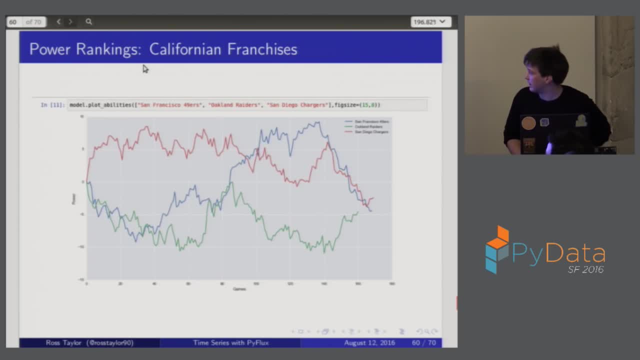 but never quite got it recently. California Franchisers: they used to be good, basically, But zero, by the way, means about average, So they're actually. these three teams now are below average. San Francisco were good for a while, in 2013.. 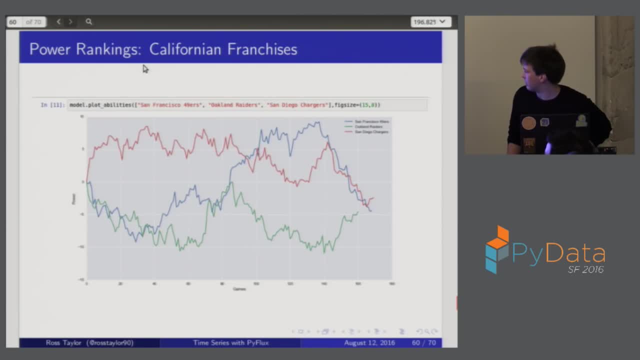 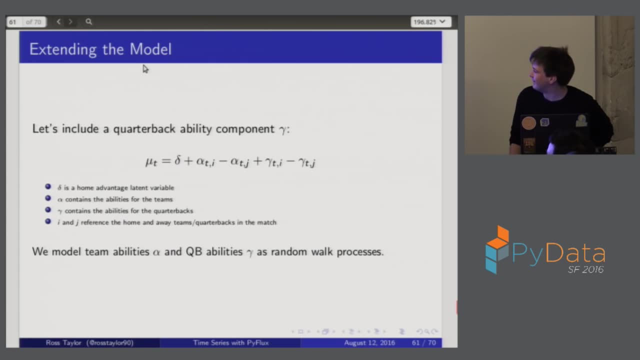 They've gone down a bit now. Oakland Raiders have been a bit bad generally. They're getting better, And the Chargers as well. This is a bit of a bleak pitch, I'm sorry about that. OK, let's extend that. 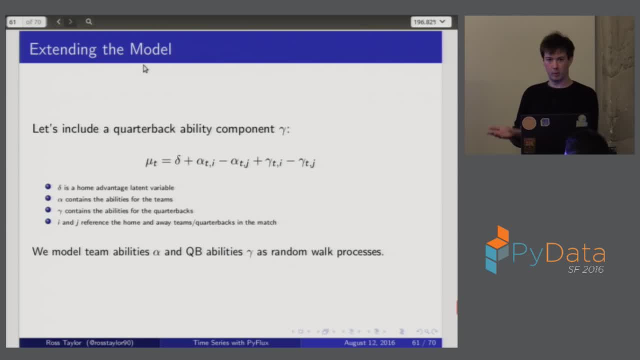 So NFL's a bit weird in the sense that there's a lot of reliance on one player, the quarterback. Now there are parallels in other sports, like soccer might have a star striker or something, But the quarterback is really weird because they're basically like a manager on the pitch. 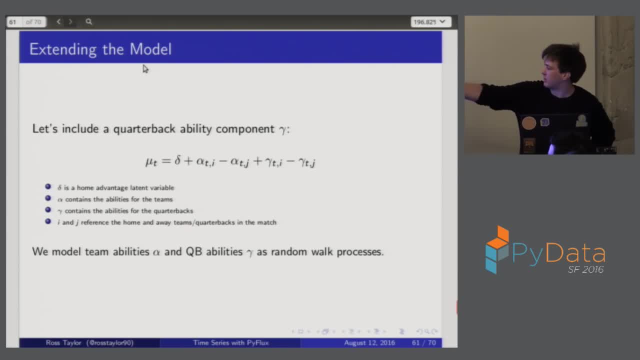 Very strange. OK, So let's have a quarterback component. So again, we've got abilities here, But now we just have another component specifying the quarterback in the match. So we're modeling it by gamma. So if it's like I don't know, Denver Broncos or some team, 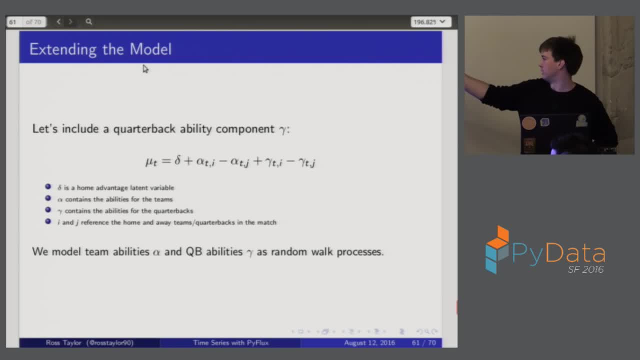 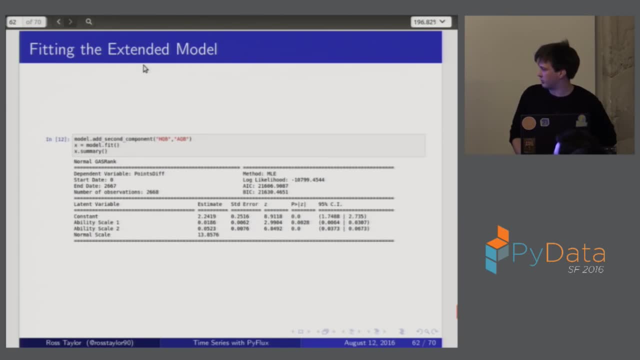 last year. then we'd have like Peyton Manning or Osweiler or whatever in that term, So it's basically exactly the same as team abilities. Now we've got a quarterback component And we're going to model it as a random walk process as well. 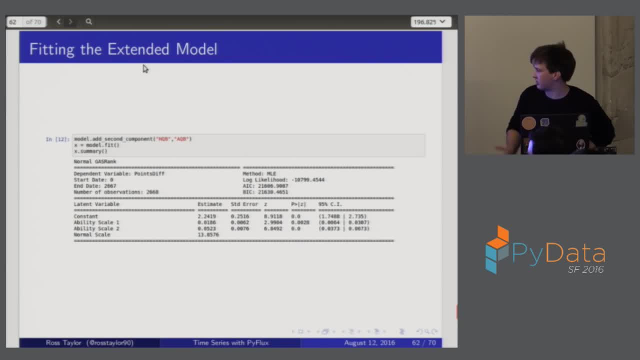 So with the same model, I've just got this easy syntax, So add a second component, So home quarterback and away quarterback And it's basically like a second term for that team, if you like. We fit the model. And let's have a look at some graphs. 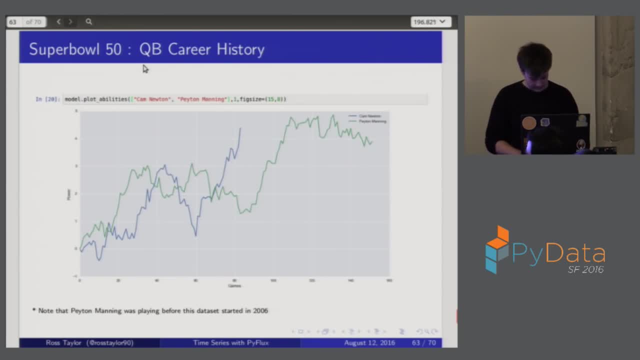 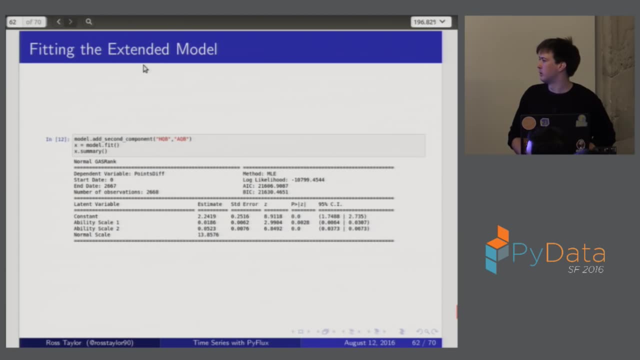 Are you just using something like Patsy as your definition? Yes, For this model. when you first specify it, you actually. no, I don't think you do in this particular model, because you've basically just defined the home and away team. 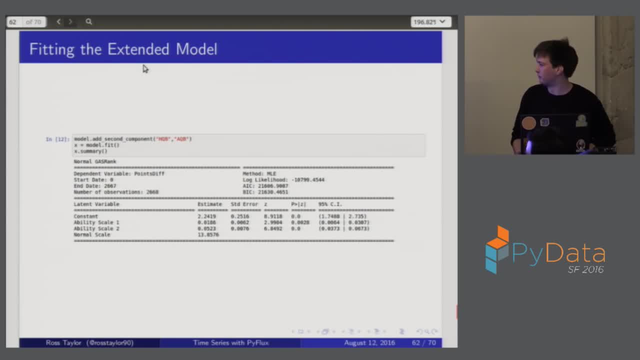 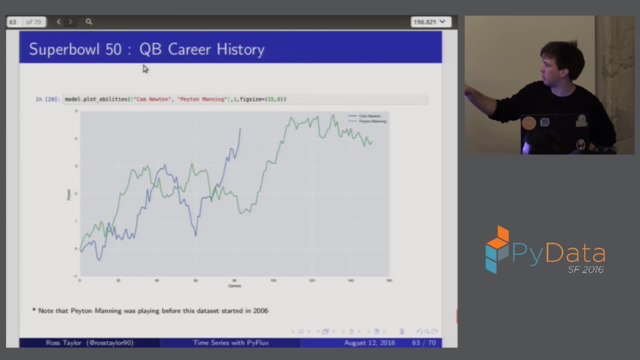 just by the strings. I probably could use Patsy or something like that. So it's a good shout, But I use Patsy elsewhere. OK, So Super Bowl 50,. you can see the career history here. It's not quite career history, because it goes back to 2006.. 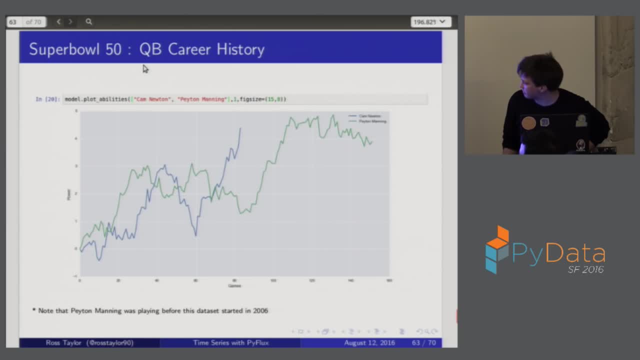 And Manning was obviously before that time. So Cam Newton obviously shot up in the last season. Peyton Manning seemed to have a late resurgent but was probably a bit on decline. The question is well, can we get uncertainty? 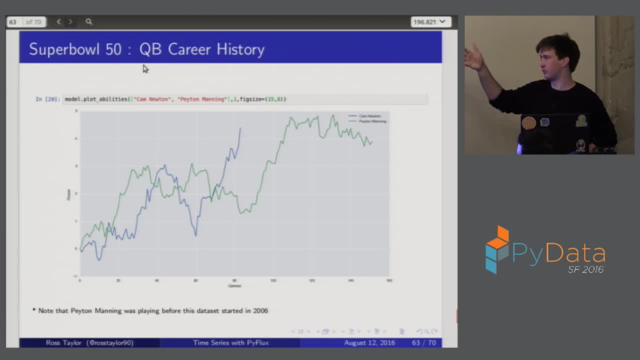 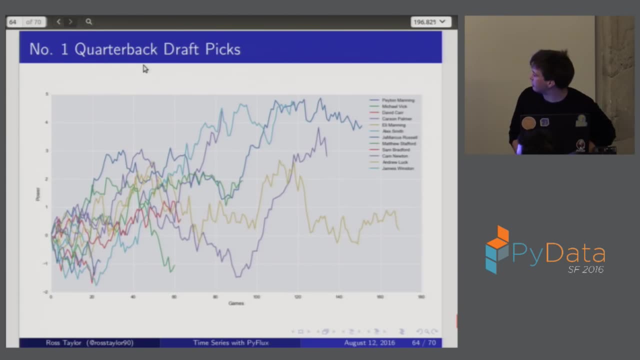 for these kind of things. What would the confidence bounce You can? You basically have to just know the uncertainty of the learning rate term. But anyway, the point is there's two quarterbacks. You can also do things like fun, So look at no one quarterback draft picks. 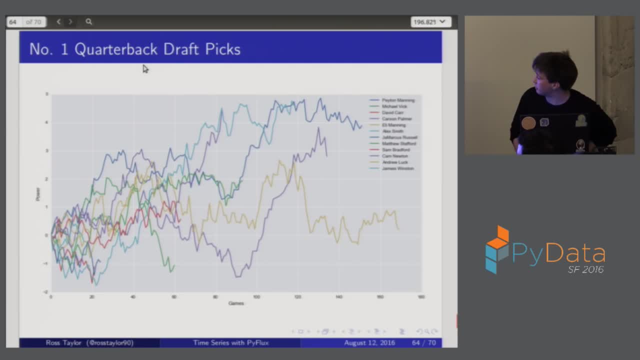 So the top. there is Peyton Manning again. Alex Smith is also particularly like this model. He's the light blue up there. Carson Palmer is in the purple. He's had a resurgence. LA Manning has been OK-ish, probably a bit better than average. 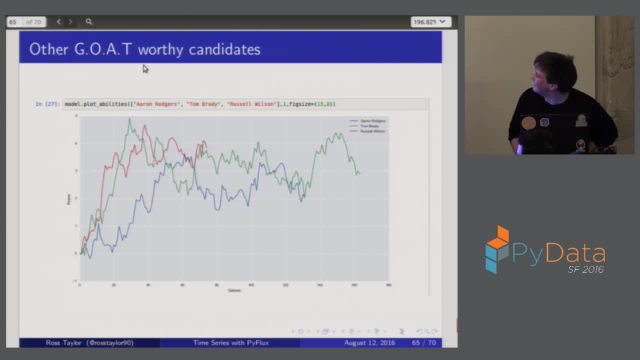 Michael Vick- let's not talk about that- And other guys- And this is going to get into the limitations of this model a bit. I mean, Tom Brady's obviously an amazing quarterback, So that's fine, And Russell Wilson is as well. 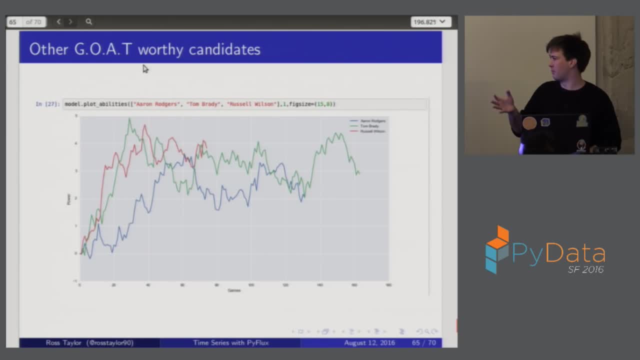 But someone like Aaron Rodgers. So basically, I did sports prediction for a bit And we always have these examples of players that aren't quite picked up by basic models. In soccer, the example is like Mesut Ozil, who's like a player for Arsenal. 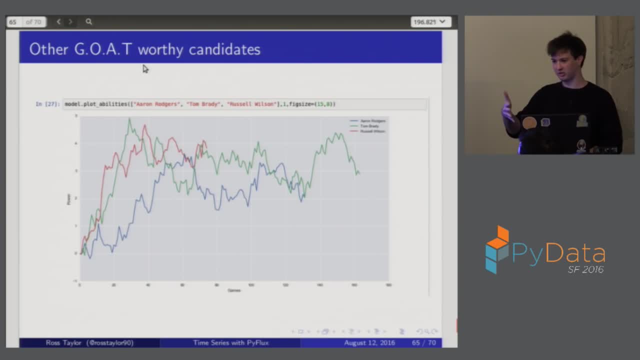 He's an incredible player, but you don't quite pick up his contribution by looking at basic stats, And Aaron Rodgers is kind of similar in this respect. I mean, it definitely picks him up as a good quarterback, but not say like top three or something like that. 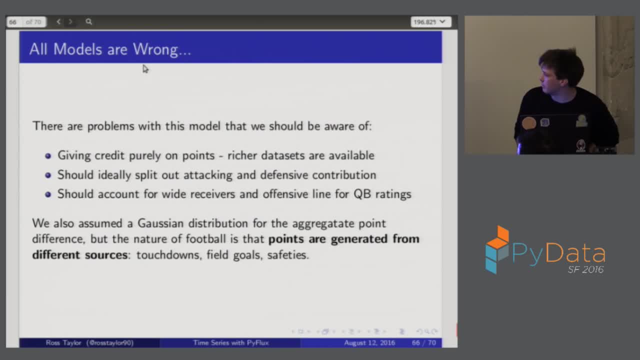 But that's potentially wrong. So let's go, Let's quickly review that All models are wrong. So we're giving credits purely on points. There are rich data sets available. We have information on punts like net pass yards, all this kind of stuff. 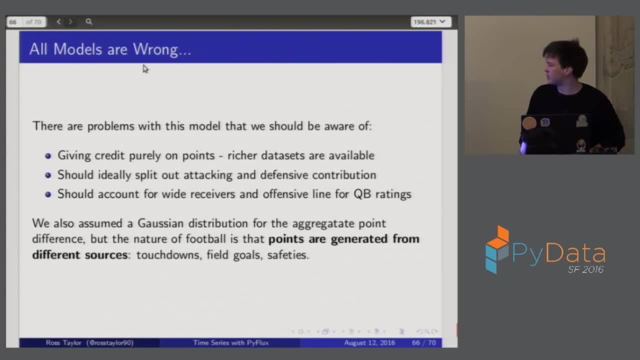 And also just detailed in-game data as well. The other thing is we've just assumed power ratings for the point difference, But what we really want here is like attacking and defensive contribution as well, as I'll show in a bit. And also we've just got a quarterback component. 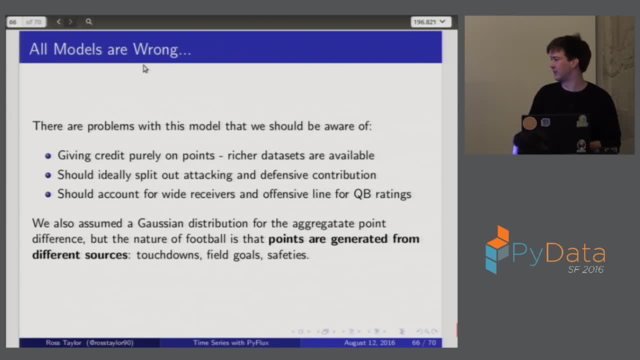 But quarterback performance is heavily dependent on things like the quality of your wide receivers if they make a catch, and your offensive line. And a more general point: if you just want to make, if you yourself want to make more complex models, it's like think about the nature of football. 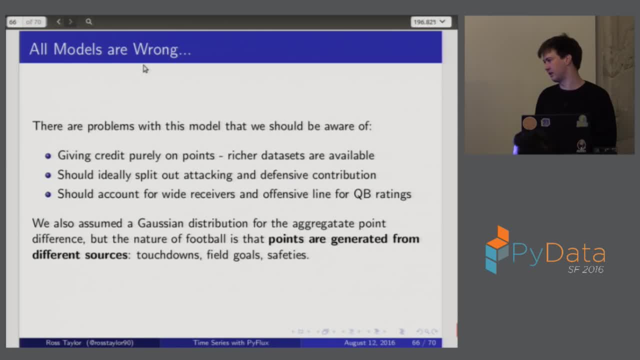 Like points are generated from different sources: Touchdowns, field goals, safeties- I mean there's a common component there in that you progress up the pitch so that makes you more likely to get a touchdown than a field goal. But that's a limitation of just doing a simple model. So Aaron Rodgers, for example, had not a good year last year, but probably wasn't his fault. He still had some amazing moments like Hail Marys and stuff, But his offensive line wasn't that great. And then Jordy Nelson, who was their star wide receiver. 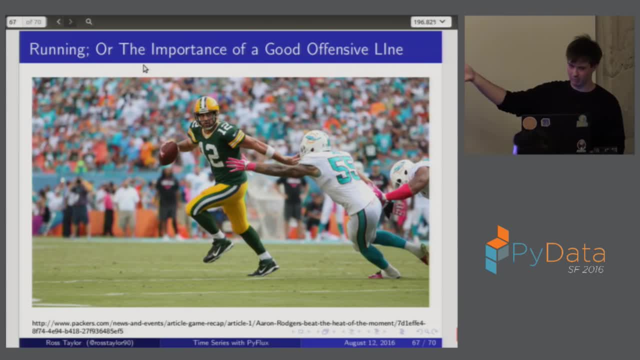 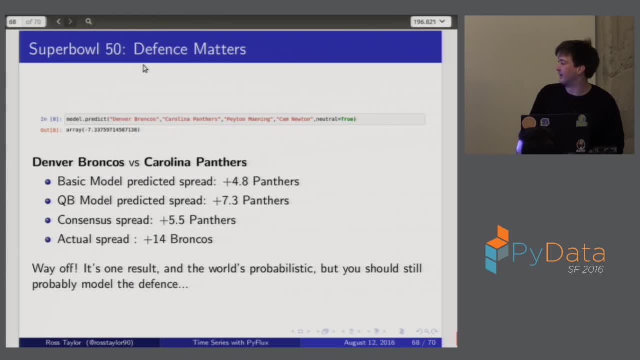 got put out. So this model doesn't take that into account. So it wouldn't really like him that much. But that's not technically right And defense matters. So for fun, I just got the consensus point spread for the Super Bowl last year. 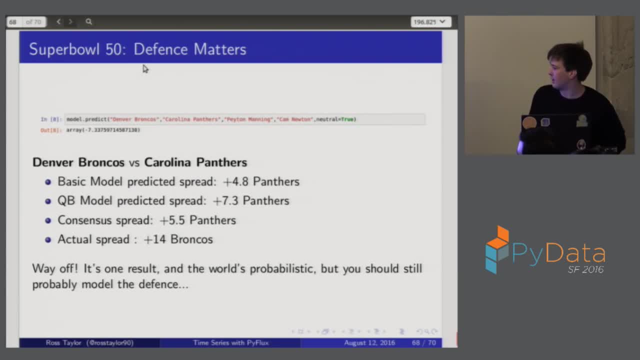 So everyone was heavily on the Panthers And I've just got the two models here And basically the market and these two basic models completely wrong, Like the Broncos like smashed it And they did it because they had like 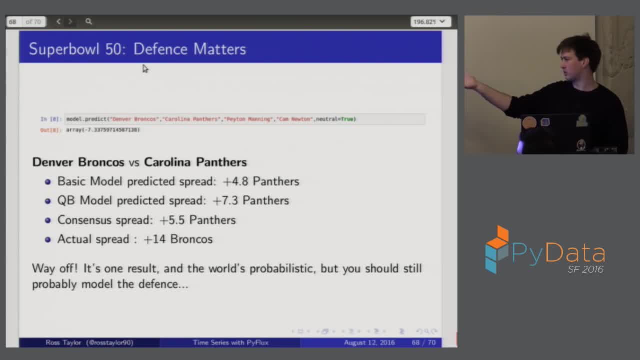 a really world-class like defensive performance, And that's a limitation of the model. Now what you could say is: well, look the world's probabilistic. Maybe you know that is the right expectation, but it just happened to go that particular way. 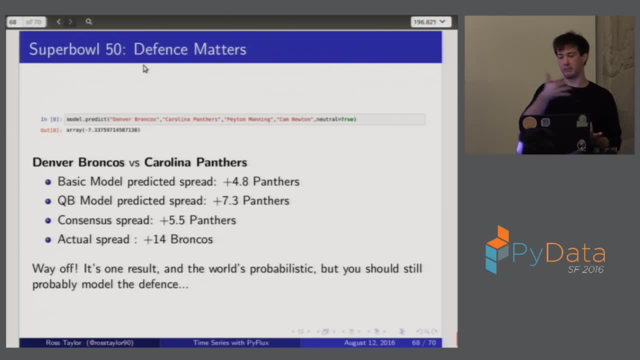 Like if someone hadn't done some certain thing in the match, then perhaps, like the Panthers, would get some momentum or something like that. But you've still got to use your intuition a bit, Like you should probably model the defense. 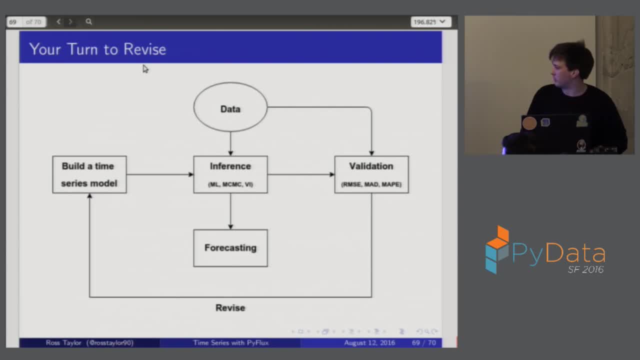 And I'm going to finish using Boxer's Loop. So again I've shown you some models. I've mainly focused on the modeling bit, touched a bit on the inference- not much on validation but something to look at. But hopefully that's given you some good ideas. 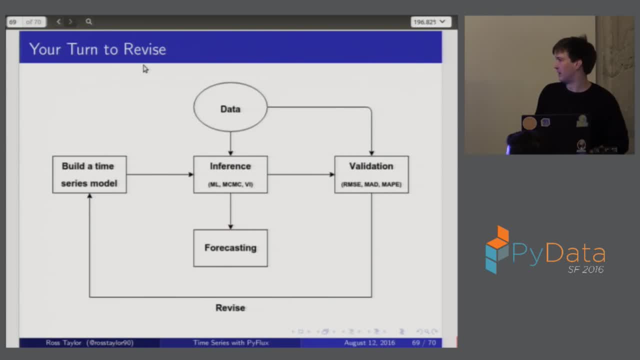 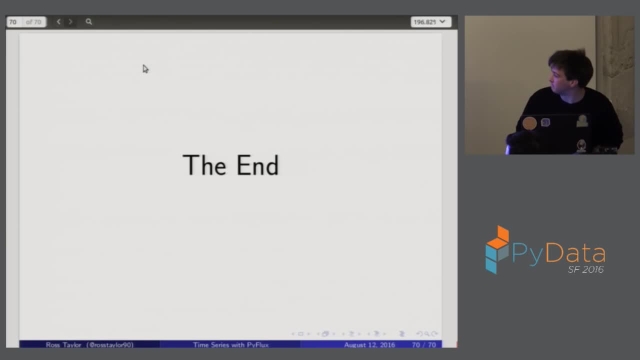 yourself to like try things out on, like finance or sports or whatever, And it's also just given you like a brief tour of the kind of models we can use to model, like time-varying behavior. Thank you very much. 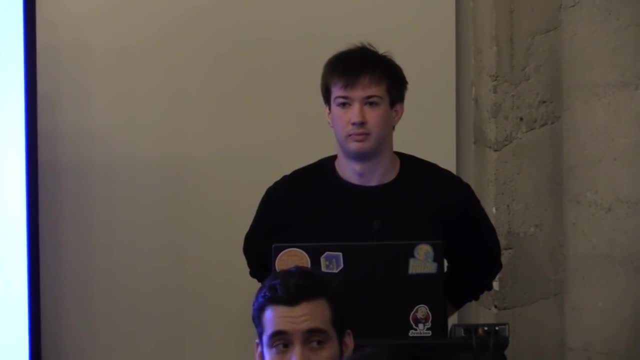 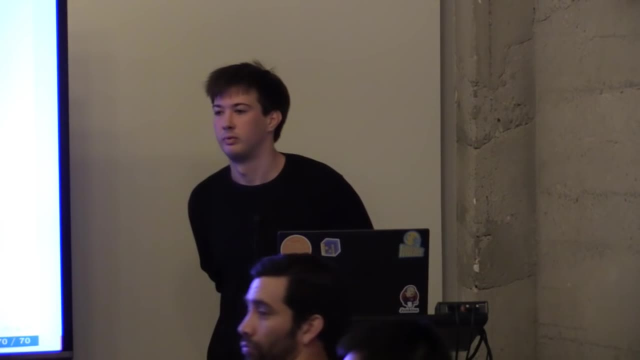 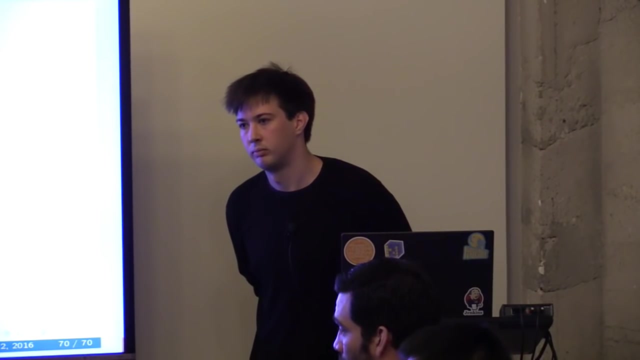 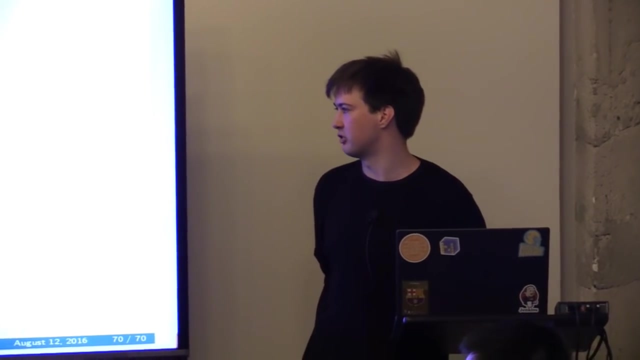 And happy to take questions. Come on, Yeah, Yeah. So like you can do like more complicated stuff and like increase the state space, Like there's things like the curse of dimensionality and stuff. But even with that, I think it's a good idea to go back and look at the basic ideas. 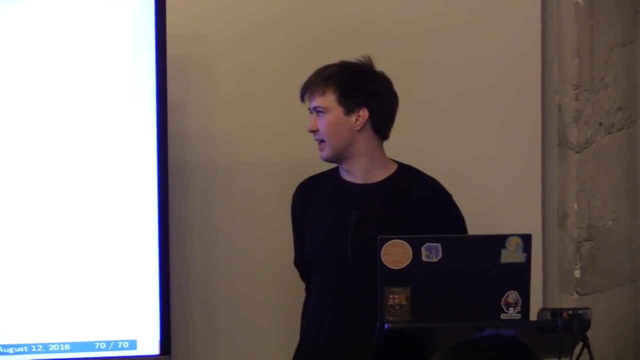 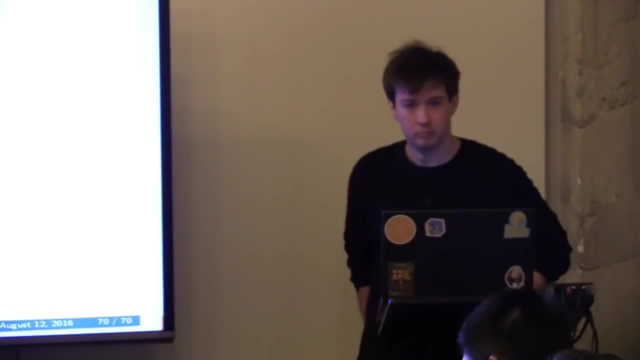 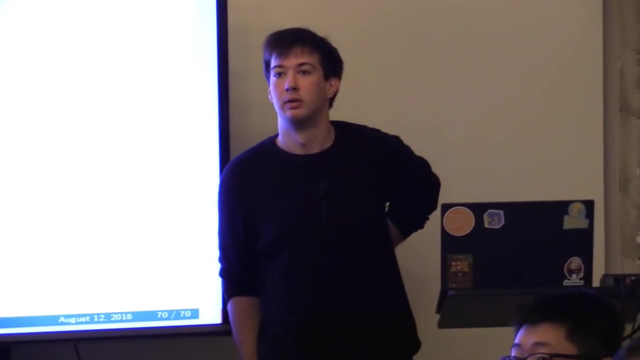 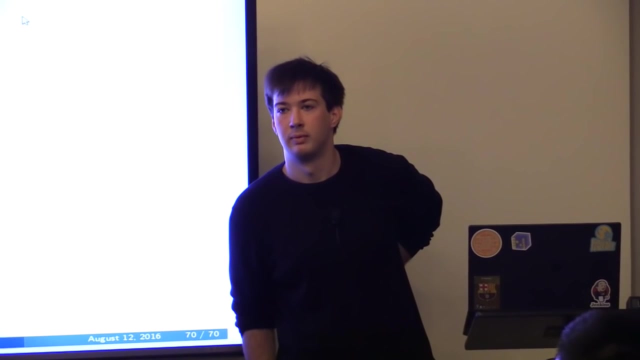 You should be worried about, and that links to the point about overfitting. But yeah, like this data set, you could do a lot more of that. I've shown like a very simple model. Yeah, Yeah, Sorry, Okay, so I basically again a similar limitation. 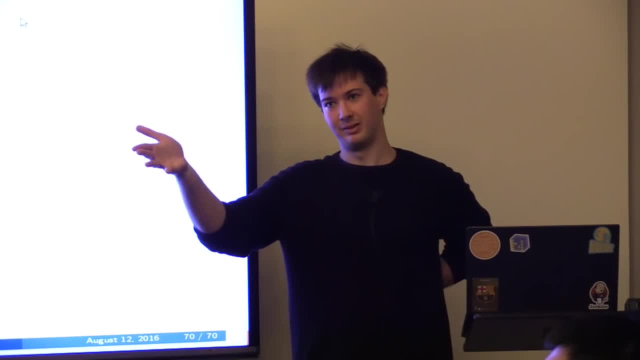 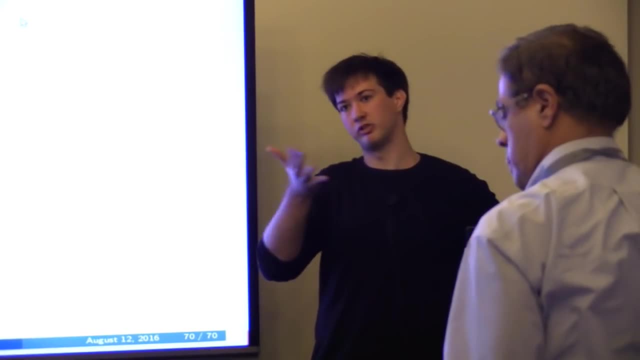 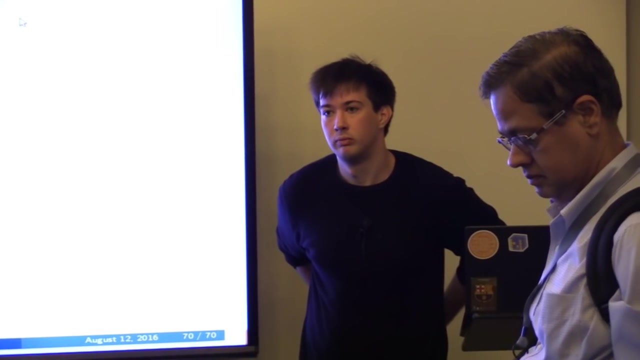 I just looked at who was the quarterback for the majority of time in that match. So yeah, Does that answer your question, or okay? So that's a lesson limitation, right, If you were take quarterbacks or something you may? yeah, Sport spending is illegal in the US and I work in finance, not sports bank, So 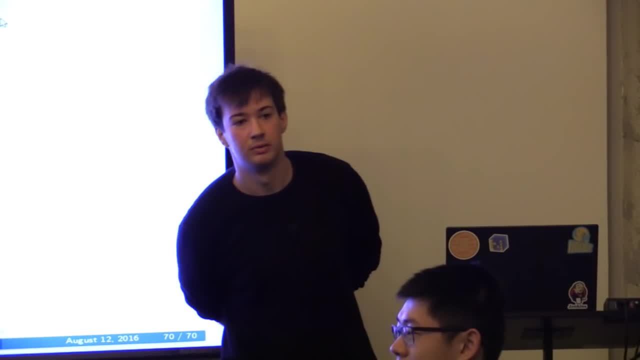 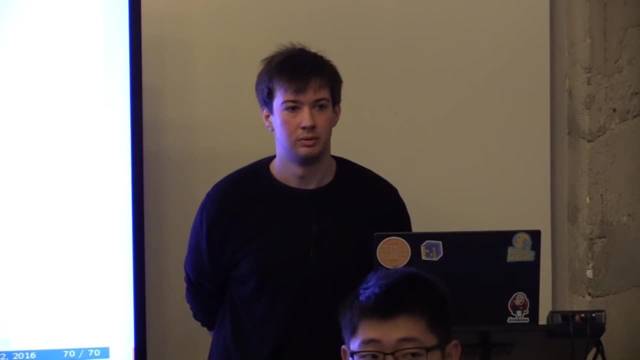 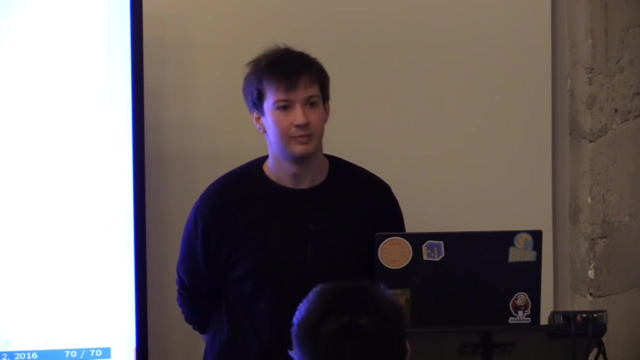 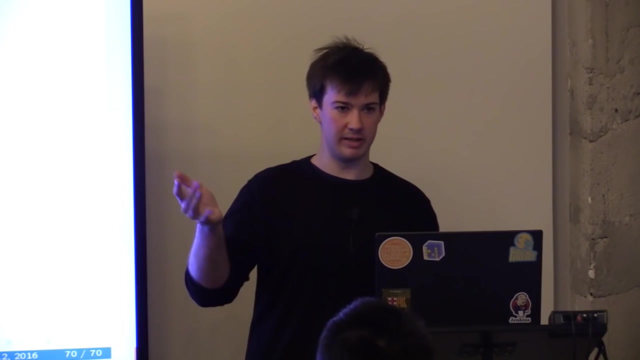 Any other questions? or Yeah, Yeah, that's a good question. so I Guess there's a number ways to do that. First of all, you just look at classic in model fit things like the likelihood, AICs, BICs. What you're probably interested in is like using a holdout period and then 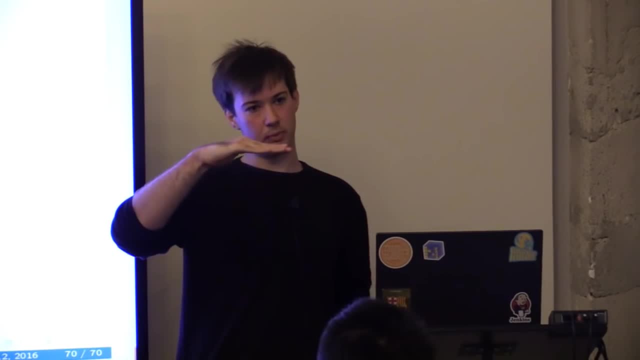 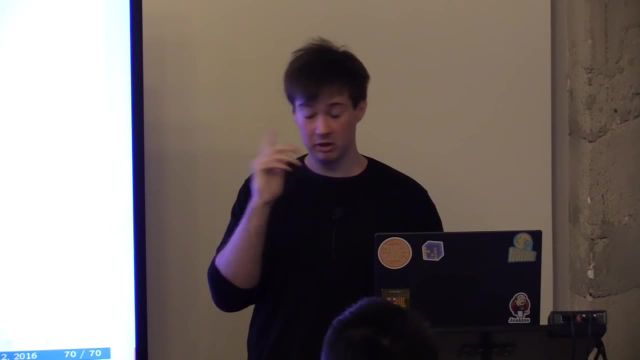 Trying to test the effect of it adding a component. So you might start with something simple, like I've done here, then gradually build on components and see what the best level of complexity is. But you know there are some problems with that. to be honest, like You'll find, often the times, if you look it's like certain, like periods in, like the history of a sport and certain things are more. 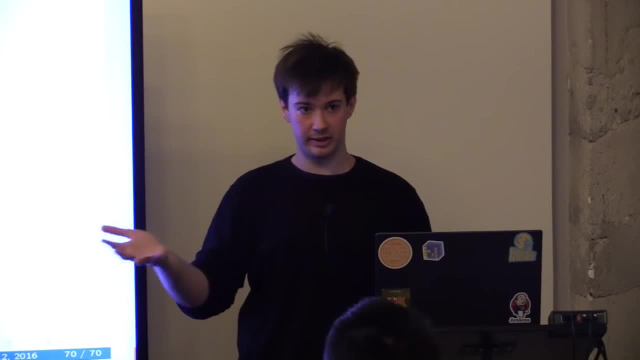 Predictive and not, and the nature of the sport changes as well, Not just because of rule changes by other things. So like soccer, for example, is like notorious for that, like the style of football just changes very rapidly over decades. So there's a serious question about there, about, like what period of data is actually valuable? 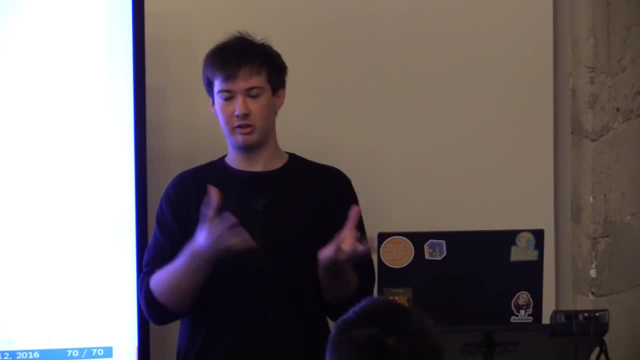 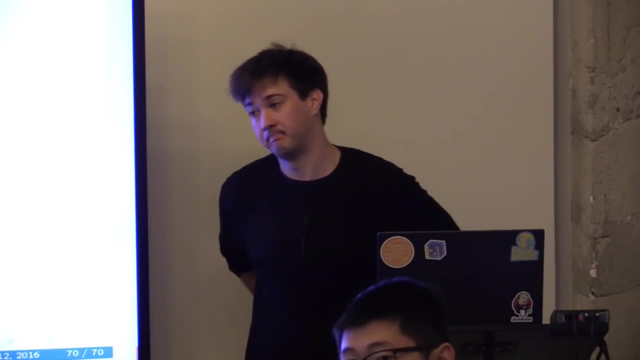 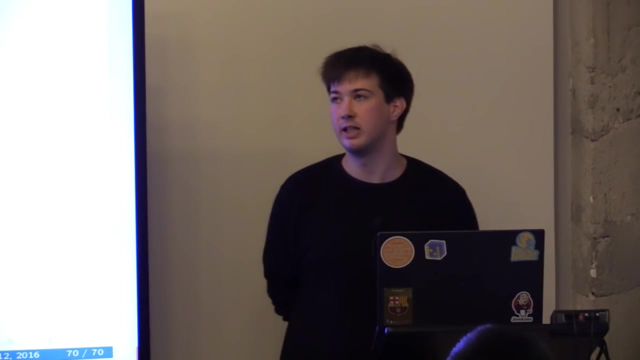 So predictive power, I guess you can't reduce it to like using a holdout period. You've got to think about a bit more. Yeah, Anyone else? Okay, so stationarity is so if you take a box, Jenkins approached and you care a lot about stationarity. 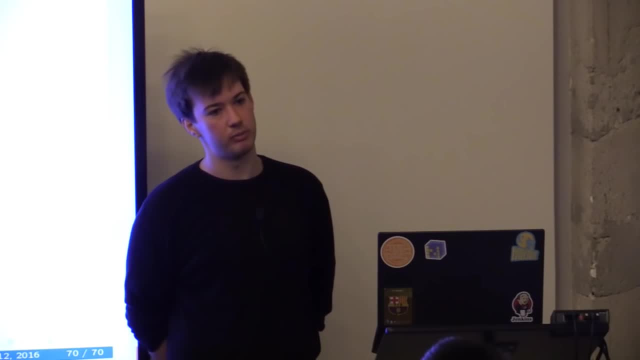 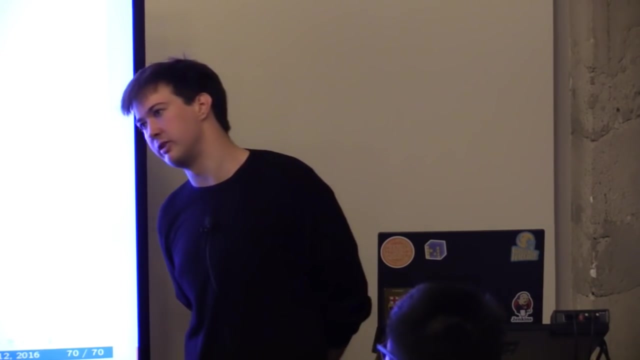 You take the state space model approach, You don't really care because it's already like implicitly in the model Here us. Sure, Yeah, somebody made many using numpy and about pandas as well, just to do the data formatting. I've also just put in some like siphon in some areas to speed up bottlenecks a bit. 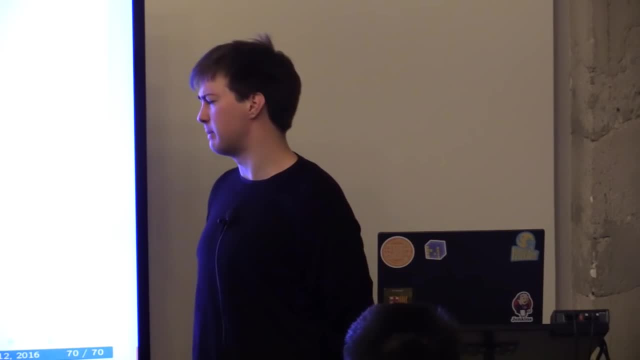 But yeah, it's basically pure numpy. There are some light limitations to the performance side that I want to address a bit, because the trouble of time series data is that You can't really avoid for loops in a lot of places. I mean the easy answer to say: well, you know, put it into siphon or something. 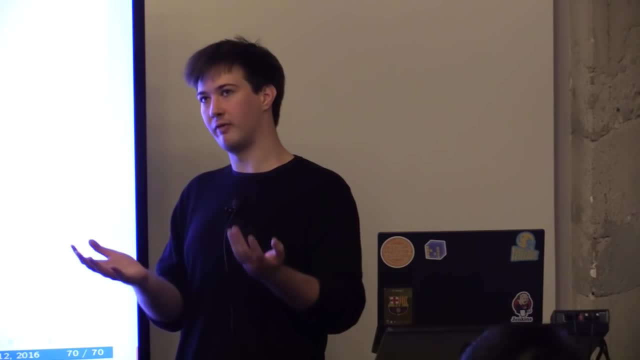 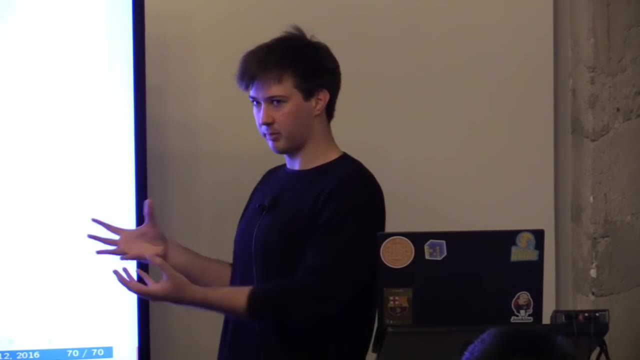 But then you also care about in a lot of cases, like having support for like custom things that the user can put in. So I've show you the gas model here. You can actually put in a custom family if you just write it in the same format, Whereas if I try to move it to like a siphon based format in that particular instance. 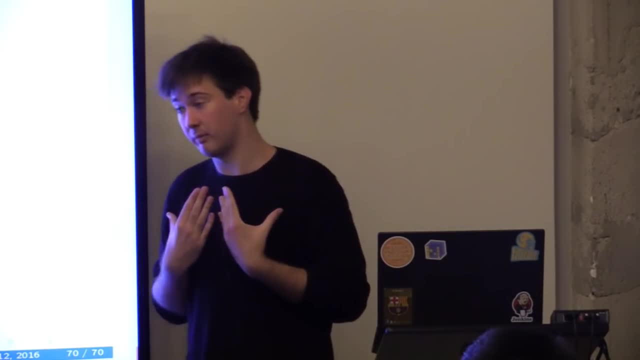 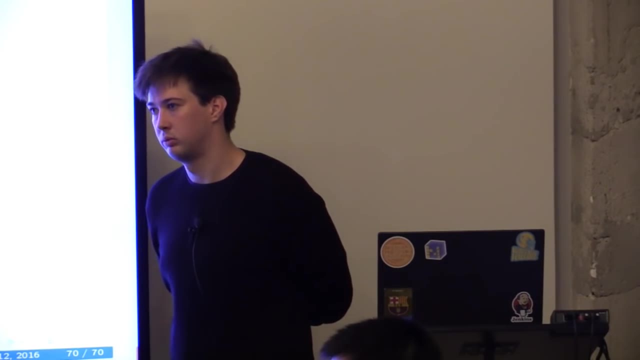 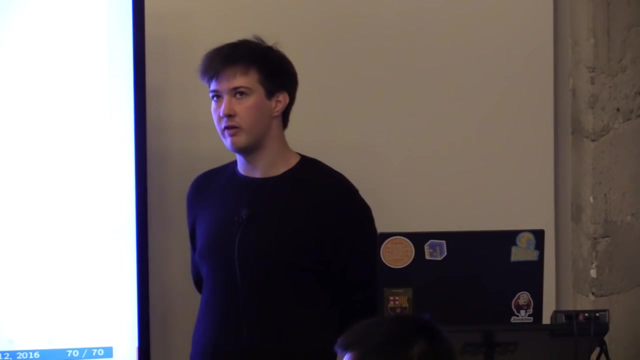 It would kind of lose the flexibility a bit. So there's a trade-off that I'm trying to bounce myself about what the best approach is, But it's mainly numpy and a bit siphon. So the big overlap is probably with stats models, Which has things like RMS bars and state space models. my own focus, to be honest, was not these types of models. 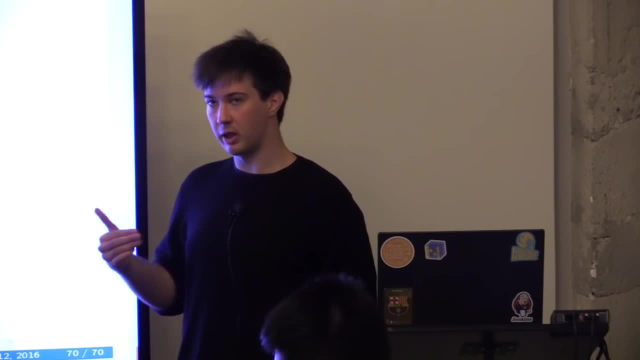 I kind of had to put them in just as building blocks for what I wanted to do, and there's my own priorities. It was these gas based models. I've also got non Gaussian models that haven't showed today, And what I'm developing now is basically more complex models based on Gaussian processes which are very useful for time series. 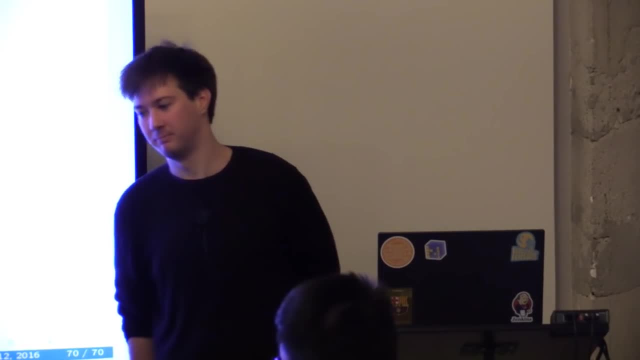 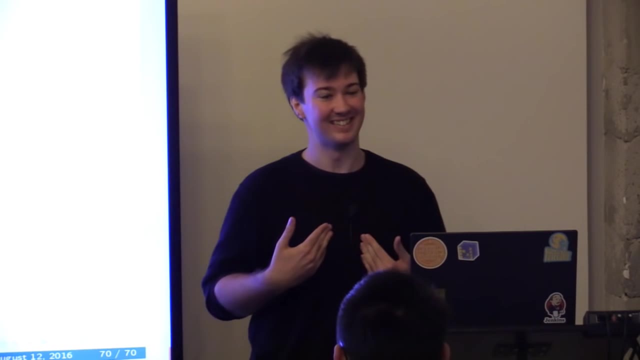 But very hard to implement the correct way. Can you tell us a little bit about how big is the 5 plus developing community? Pretty much just me right now, So it's taking up a lot of my spare time, but it's actually been very rewarding for me personally. 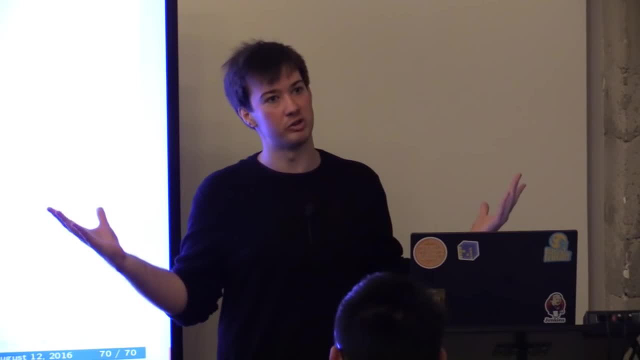 Because, like I said, I'm from a recent background. I'm still not the best guy in the world at software development, But it's been very good for me personally. I mean, if you're interested in making contributions, you're more than welcome. Like I said, I probably think it belongs somewhere else, like in stats models or something. 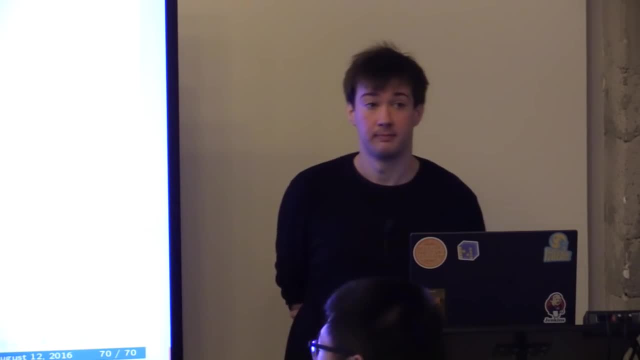 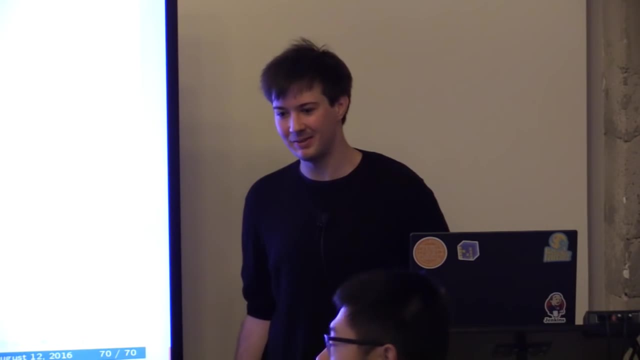 But yeah, I mean, contribution is very welcome. Yeah, How long have you been developing 5 plus Since March? Yeah, Yeah, it takes. there's a lot of, yeah, long nights. but yeah, I think I'm gonna come down a bit now and like regain a social life. 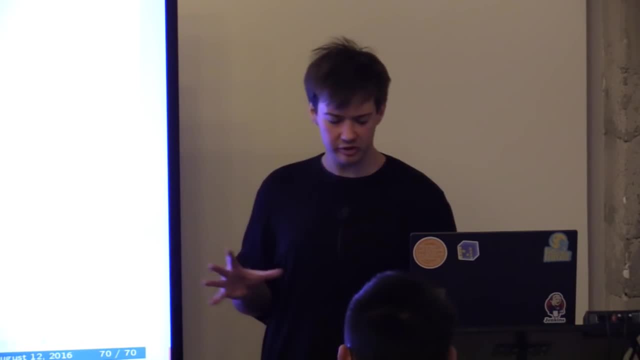 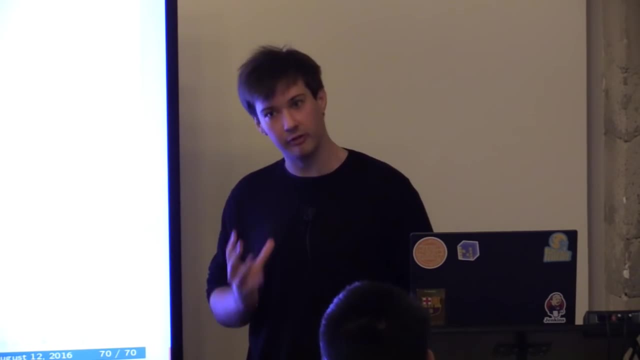 It's been very rewarding. I'd actually recommend like, Like just as a general principle if you want to like learn something in these types of models. I've done before, but the best way to actually really understand something is to actually do it yourself. Like. I can't stress that enough. It's very time-consuming and a lot of the time you'll be under pressure to like. you know. 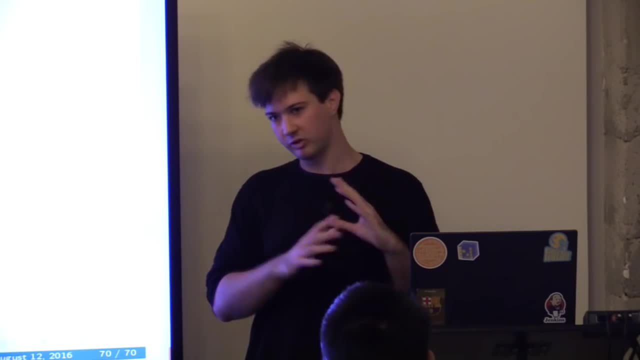 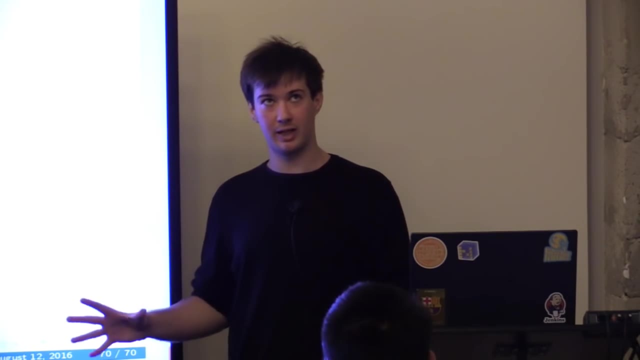 Just get a result out So you'll use a built-in library already. But seriously, like, if you're interested in you more, do with new paper, Try putting it in yourself and maybe release it as well, because it's a really good way to understand both like how the actual model itself. 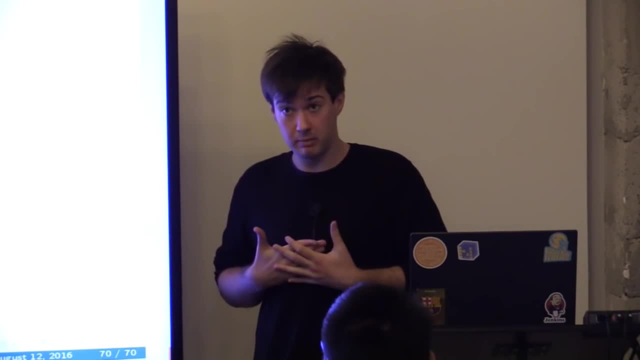 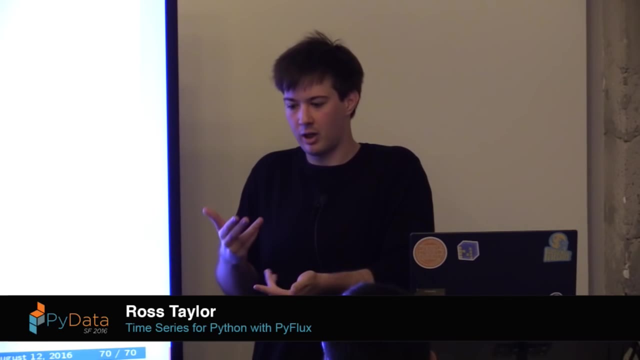 Works mathematically, but also to think about computational stuff, Like for me, like personally, something like a Gaussian process, like the maths for me is easy. And then where to put in the computational sense and the worries about things like: okay, It's very hard to invert matrices, like using like computers. I have to think about things like yeah, 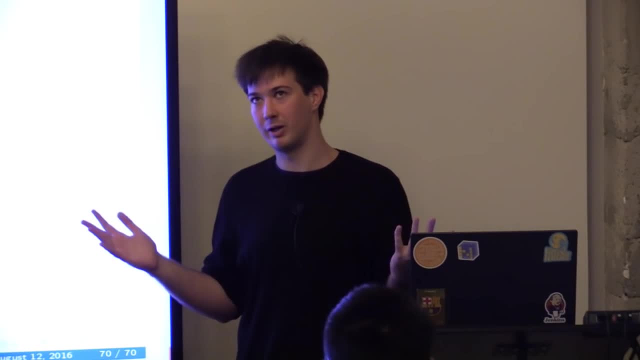 How do you? I do those kinds of things computationally right in that framework? Also, just things about like floating-point precision over rounding, like- sorry, overflow and underflow, These kind of things like I didn't have to worry about when I was doing research so much.